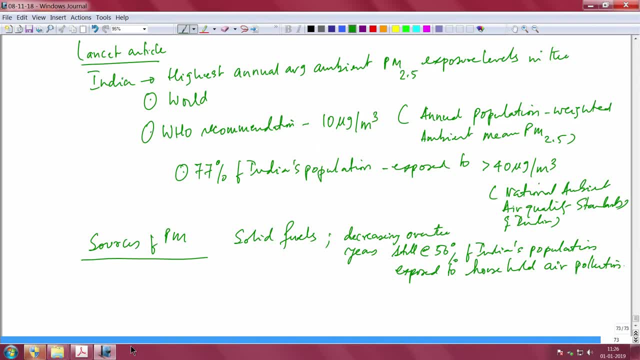 the same metric: annual population, weighted ambient mean, particulate matter 2.5.. So it is a particular matter, 2.5, but Indian standard is not saying that Indian standard comes from national ambient air quality standards of India. I have written it here and this essentially. 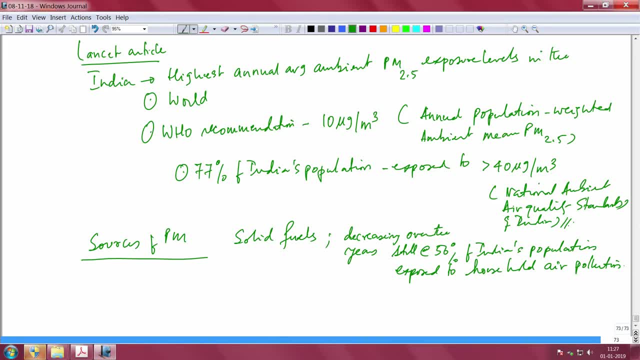 is the one that is laying the standard, and 77 percent of India's population is exposed to even the national ambient air quality standards of India, which fixes at 40 micrograms per meter cube. 77 percent, So 77 percent of India, is even greater than 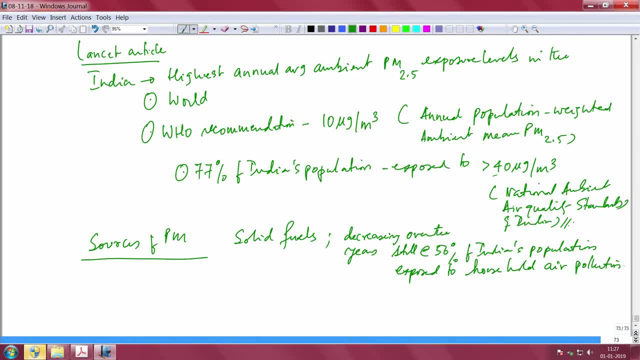 the value that is fixed by the. even by Indian standards, the value is very, very high. So 77 percent of India's population is exposed to greater than the national ambient air quality standards, which is really an issue. it means such a serious issue that you have to somehow. 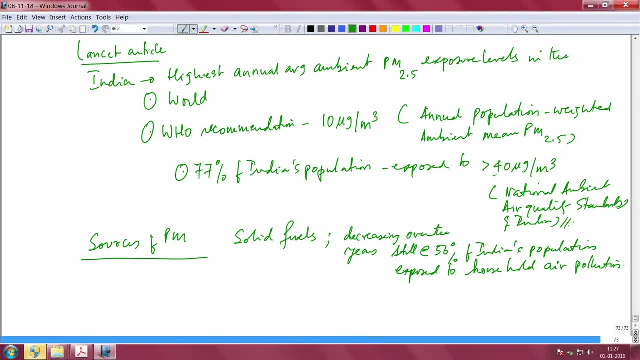 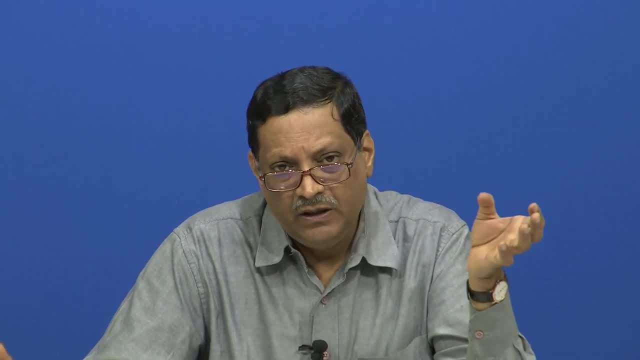 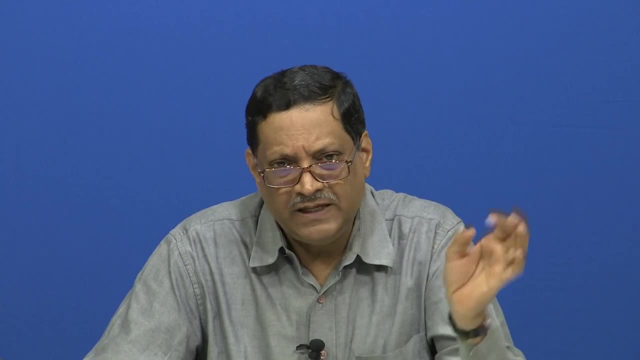 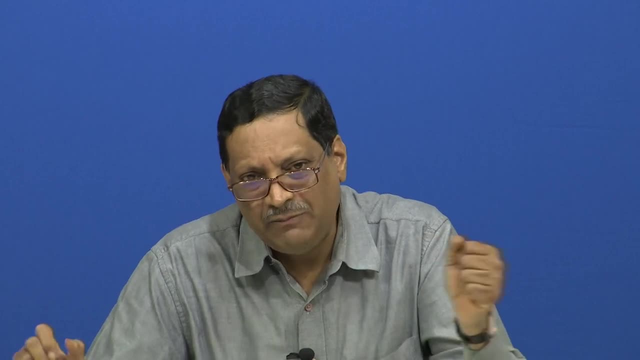 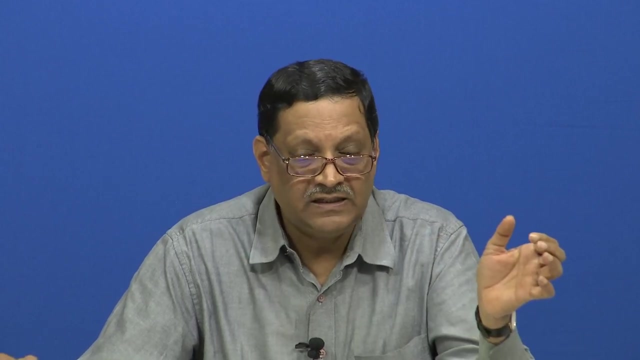 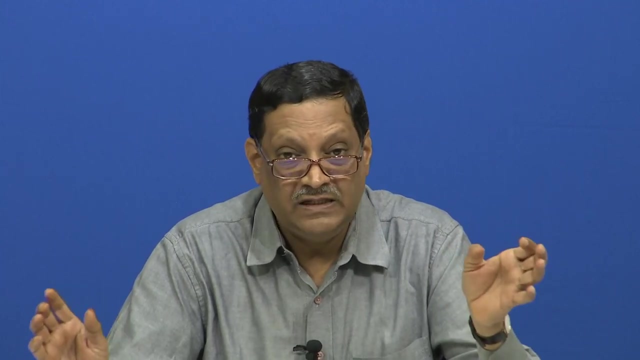 lab, which is which you know sort of, puts maximum effort in trying to design, develop and make you know air quality sensors, I think will do a great service to this country by reducing shutting down and making things very cheap for sensing and monitoring of air quality. 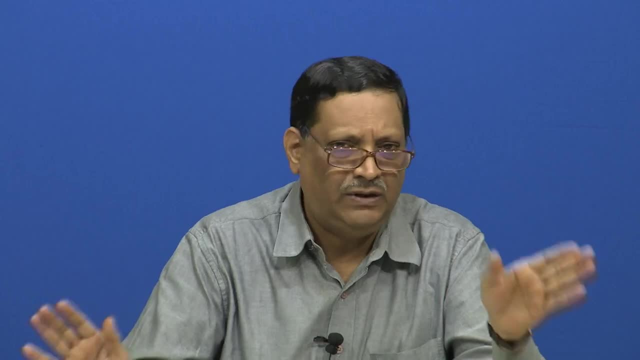 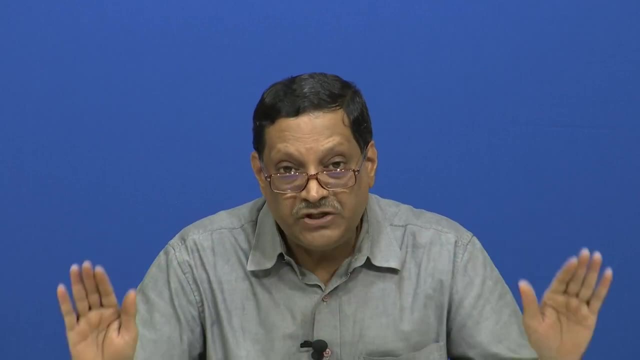 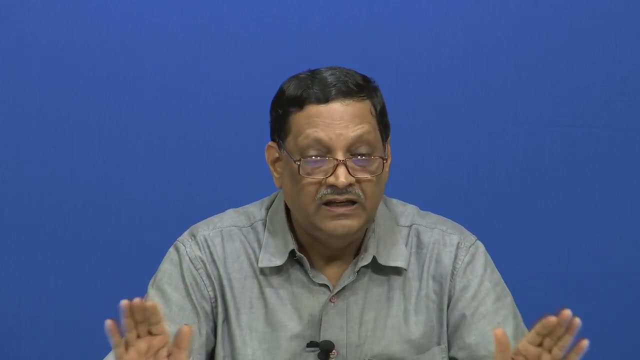 Once you know that there is an impending danger somewhere, you can do 100 different things, but first step is to actually start monitoring and give you a real feel for the special distribution of the air quality in a city, in a village, in any urban setting, rural setting, industrial. 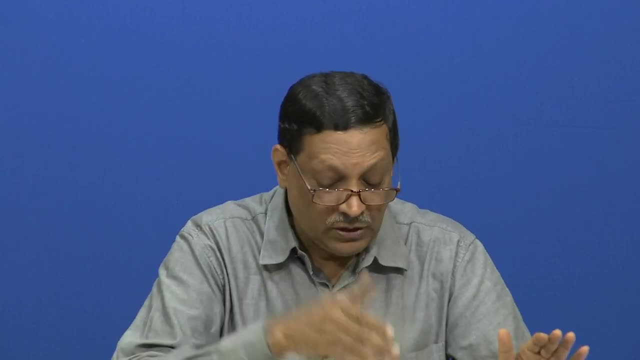 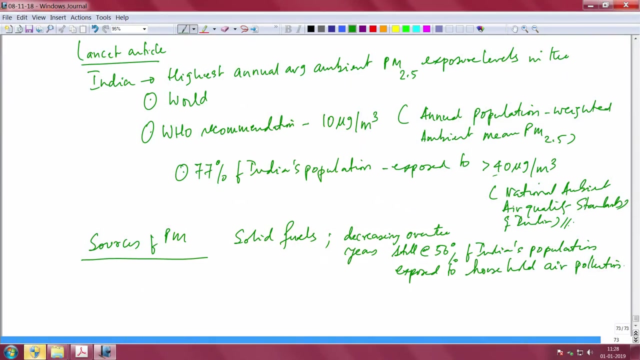 setting and all that. so this is important. So you must look at sources of particulate matter. So this article, while it is talking about particulate matter- you know what shall I say? in a way that it seems to make noise just about particulate matter. this is really not. 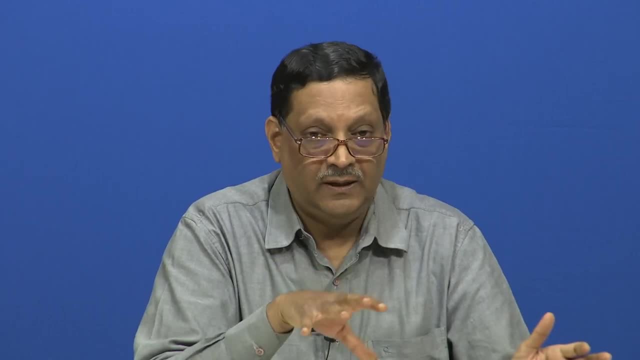 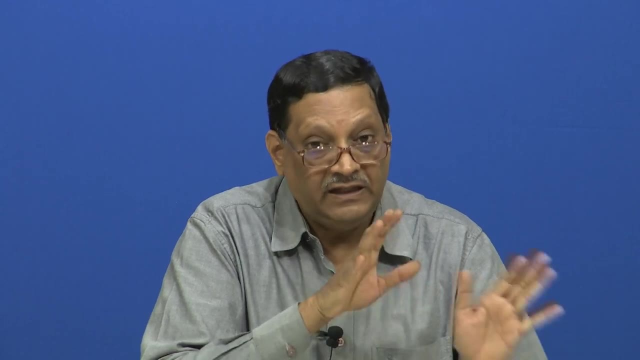 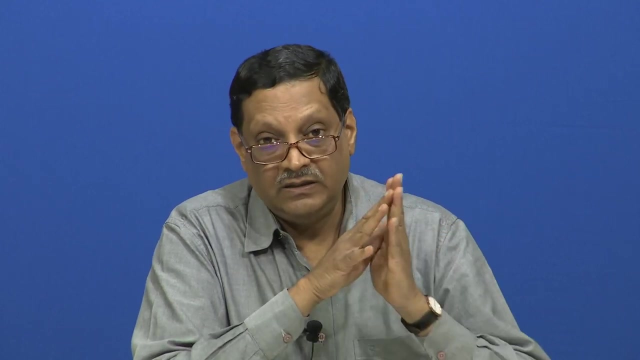 the truth. There are other elements also which are essentially causes, for you know, human suffering from air quality deaths. However, particulate matter, indeed, is a big contributor. percentage of people dying due to particulate matter is a particulate 2.5.. 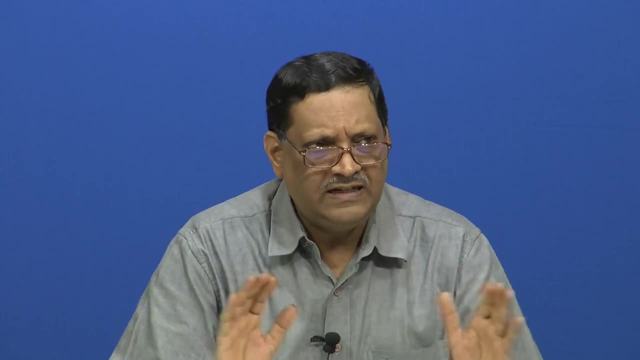 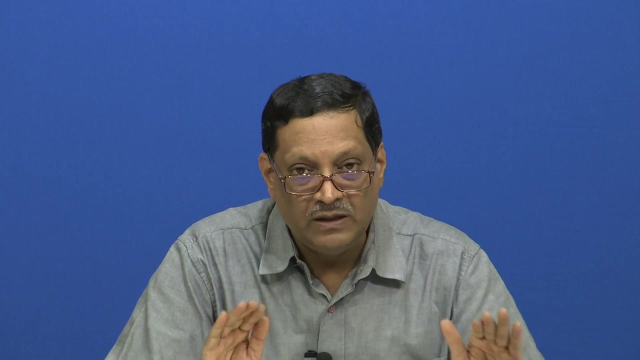 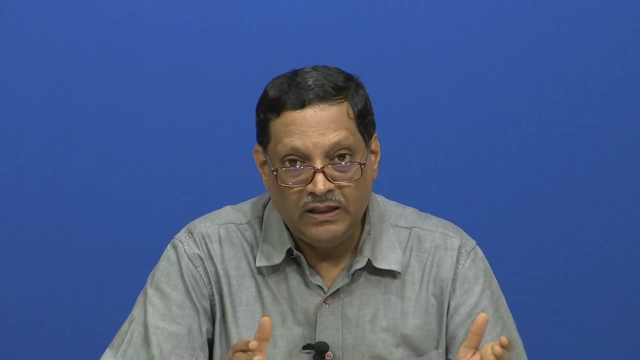 It is indeed a large number, So it is not that it is a biased opinion about this particulate matter and what happens to other air pollutants. This paper is sort of focusing more on the PM, because that appears to be the one that seems to have a maximum impact. 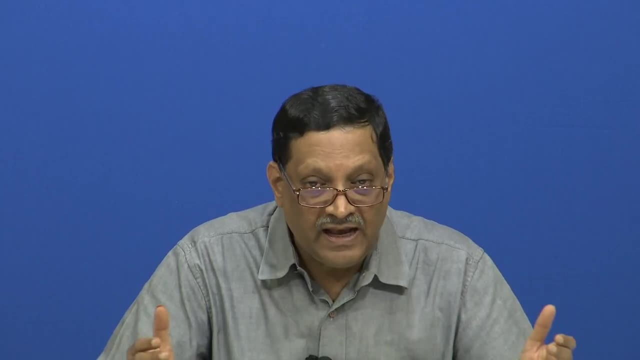 For example, it encompasses several areas from which you can look at air quality. I will come to that because this article itself is talking about that. I will have to land a take on that currently part and much No ExactlyvarGG response. 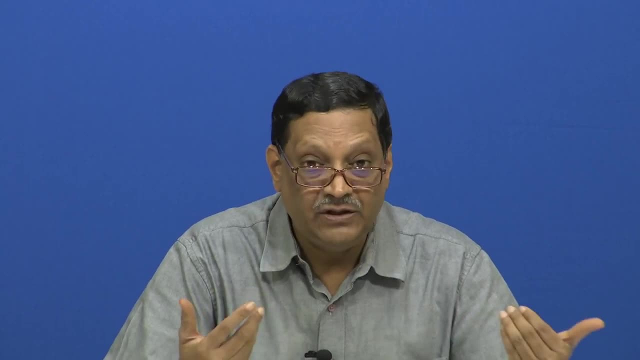 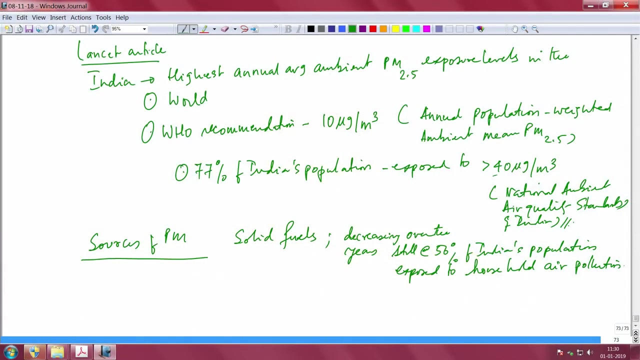 Okay, Yes, sir, Yes sir, thank you very much the mail. Okay, bye, bye, sir, No problem, take care several areas in which PM actually gets generated. First thing is solid fuels. is a is an important thing. why is this critical? because you look. 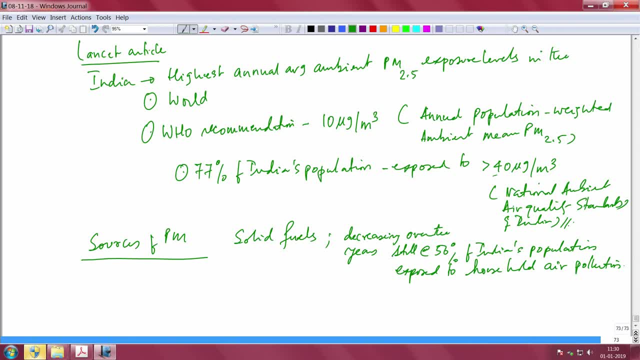 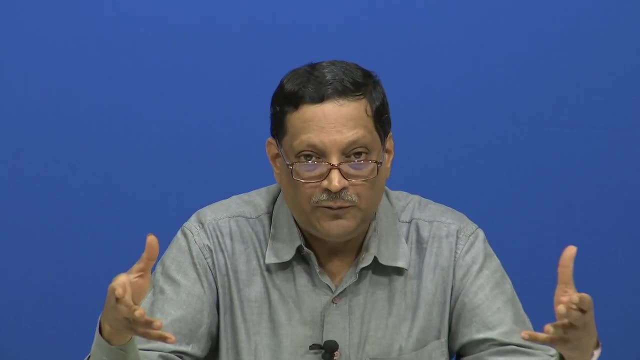 at. you know different type of efforts by several national labs and I know institutions, R and D labs and all that they come out with: what is a good stove for the village population, how to ensure that you know they do not absorb too much of smoke and which is encompassed? 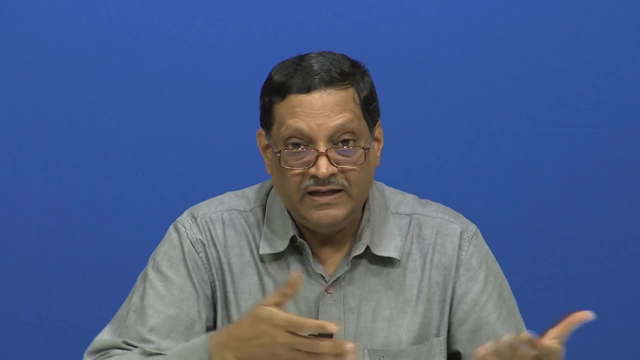 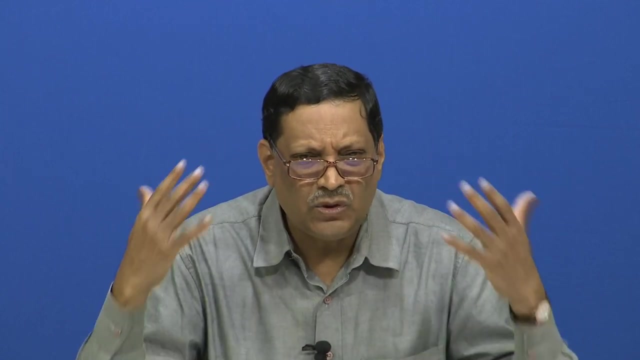 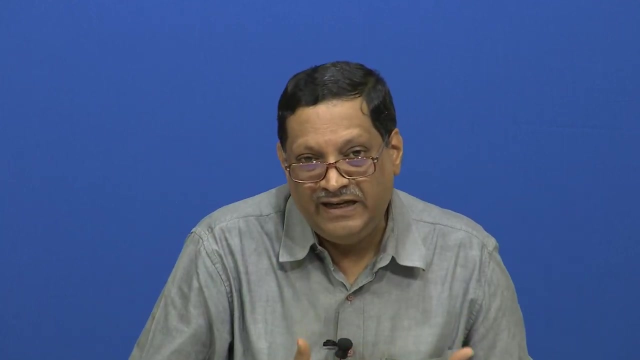 with so much of particulate matter, because you need to cook right and there is no fuel. this is the fuel essentially, solid fuels are essentially fuels for cooking and this is a source, huge source, of air pollution in households. See, if your problem starts right inside your home, even for a country like India, it is going. 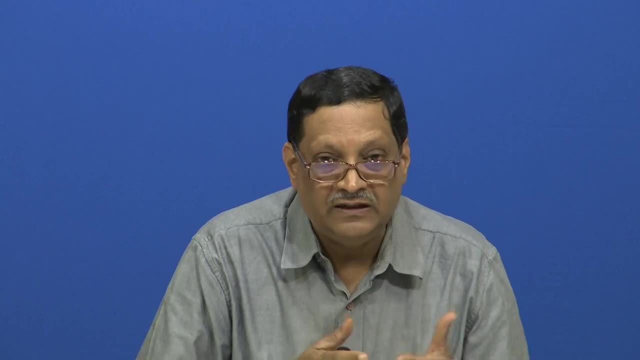 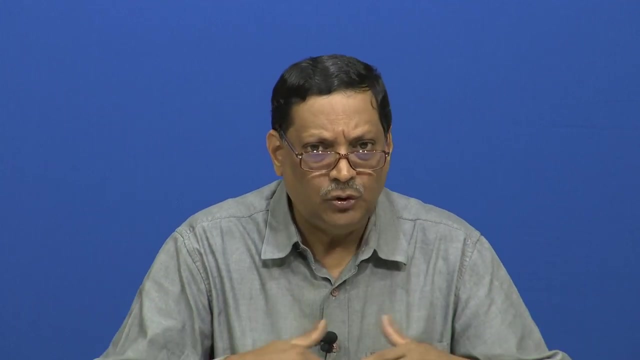 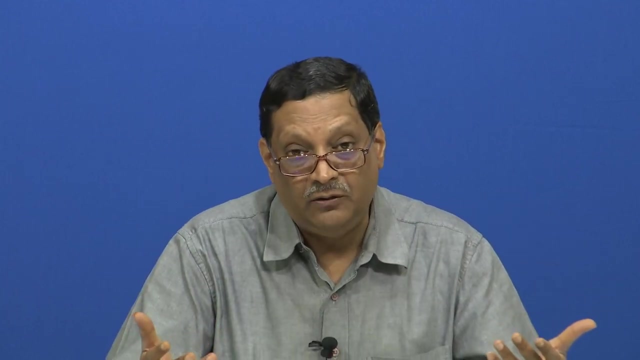 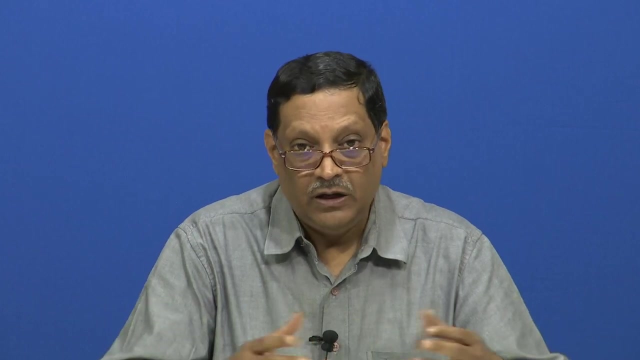 to be very hard to cut down Because you cannot monitor at the household level what you can do. therefore, major initiatives have to be taken to dispel this problem of air pollution in the country itself and therefore lot of effort has gone in trying to make you know fuel efficient, clean, energy based stoves. 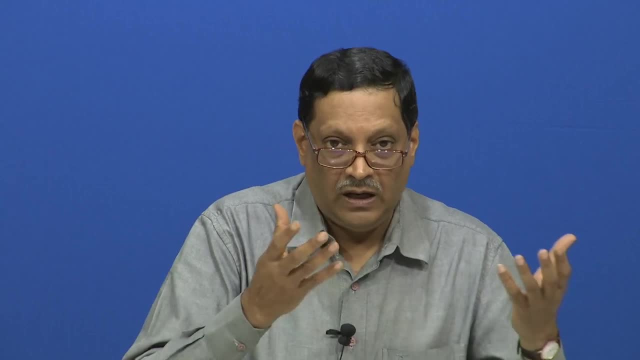 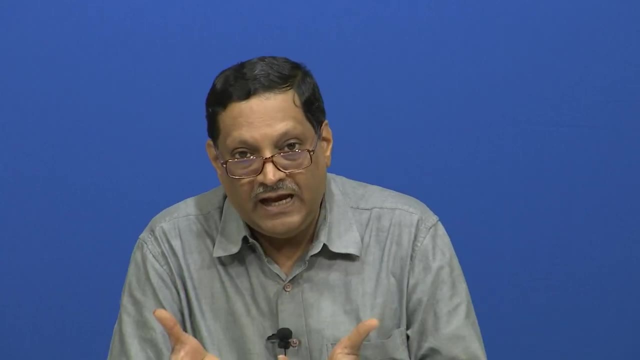 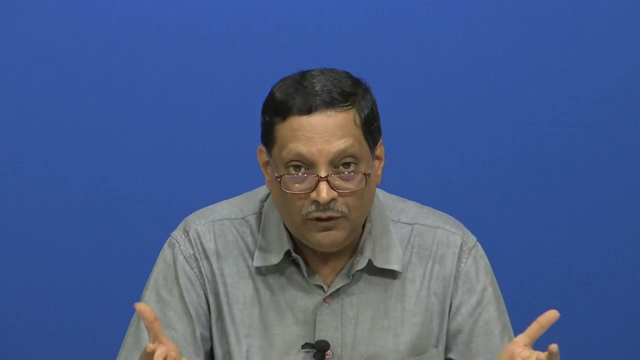 for cooking stoves, for village, for towns, for cities and so on, So, So, So what has been there? so you make it cheap, make it affordable, let people buy that and make the necessary fuel available and make create an ecosystem around the availability of fuel, clean fuel, and then people will start using it and cut down on usage of all the. 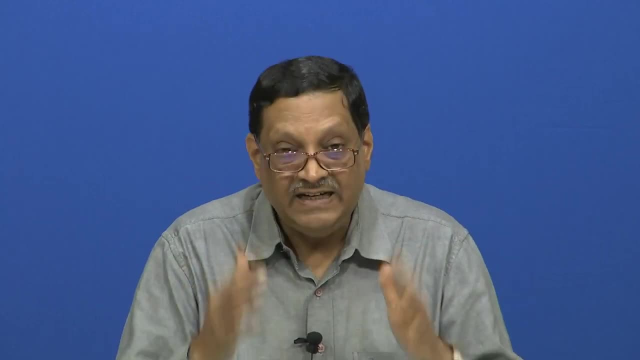 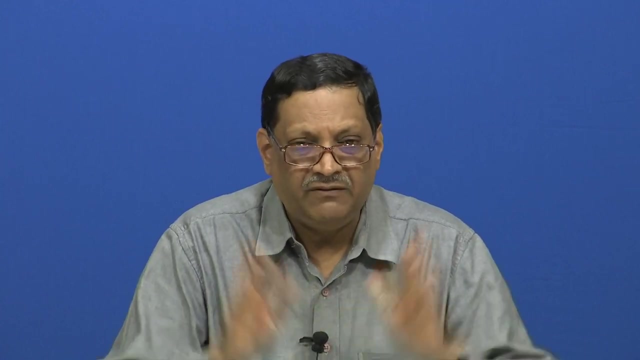 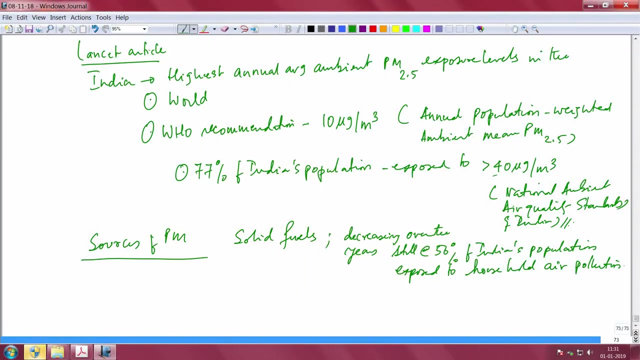 solid fuels, which essentially can be a major source. So it is decreasing. there is no doubt about it. in this country, the usage of solid fuels is coming down, but we need to do a lot more. that is the point, really. So still, 56 percent of India's population is exposed to household air pollution. this 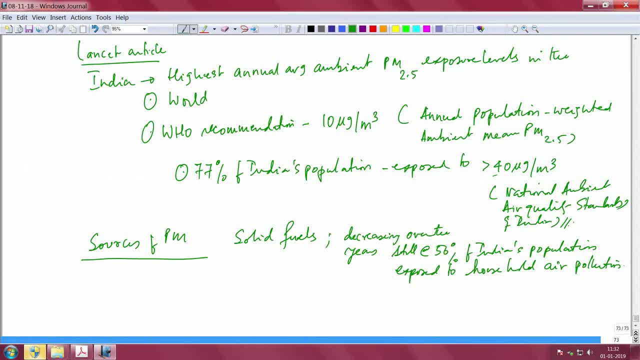 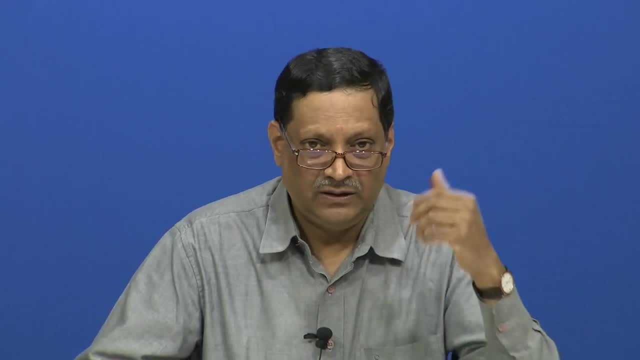 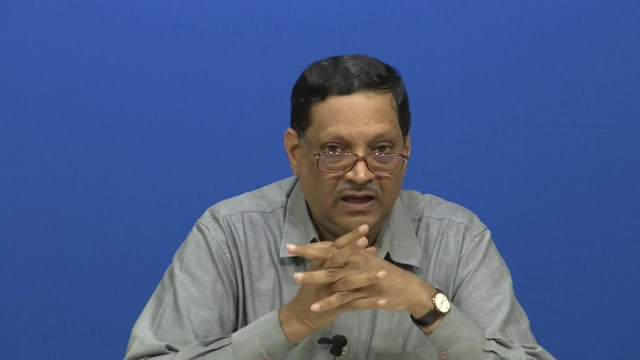 is indeed the major problem. I often go back in many years in time to let us say, 40 years back, right, So it to own a wrist watch for every individual in the house was not going to what was not really a reality, and there used to be one wrist watch and one clock in the house, and 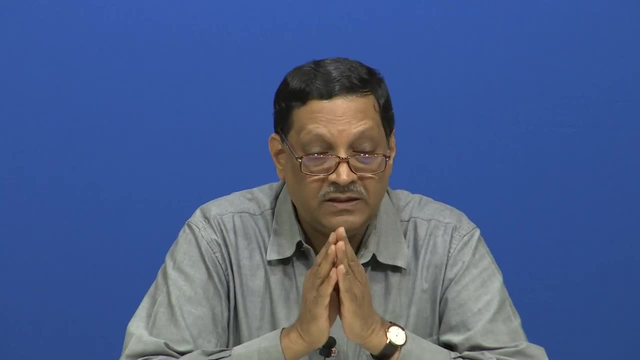 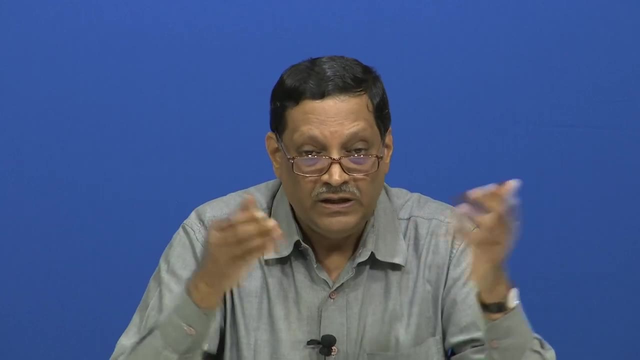 that clock. So it is a big luxury right, which means a wrist watches were very expensive. you cannot afford it. but today everyone has maybe, I do not know- 10s and 15s of watches. each time you go you buy a new model. you want to own it. it is become cheap, affordable. 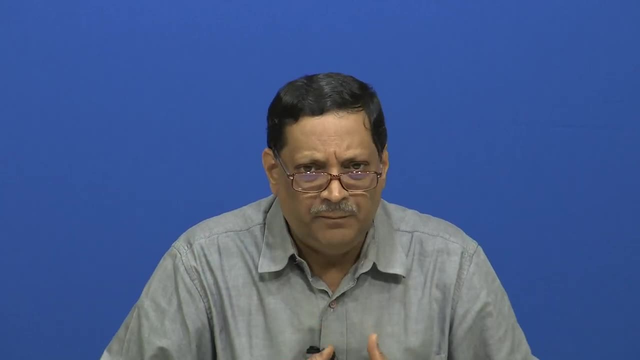 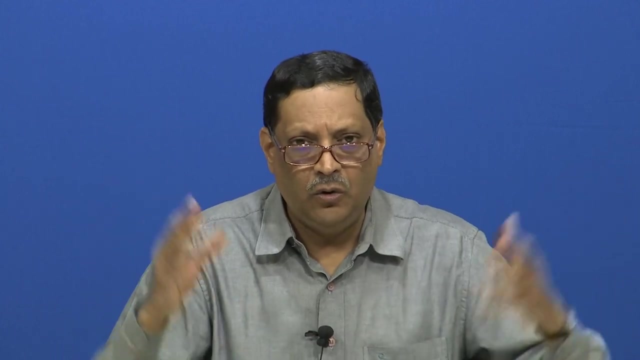 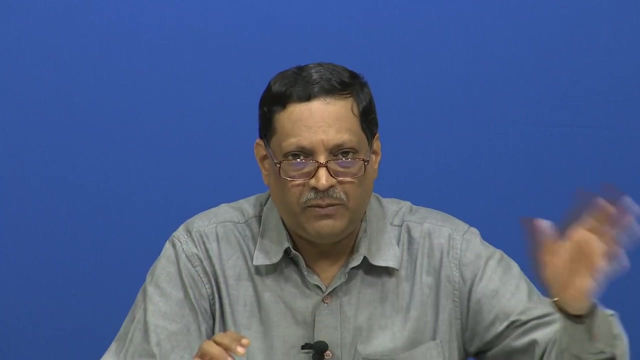 So if you can, you know, get air pollution measurement to simple devices like this and you say that wherever you go, you get a beep or a buzz and say that this is polluted here and it is So. for 100 rupees I can buy 15 rupees. I can buy a watch of that nature, although it has. 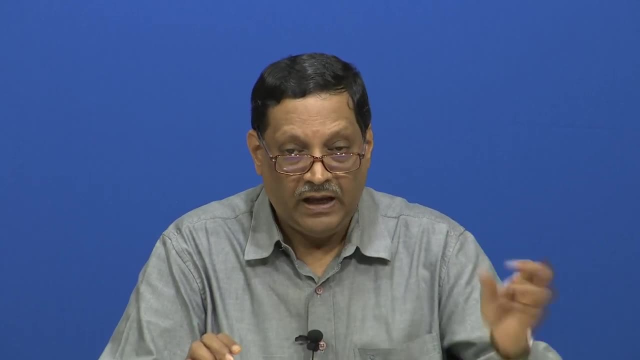 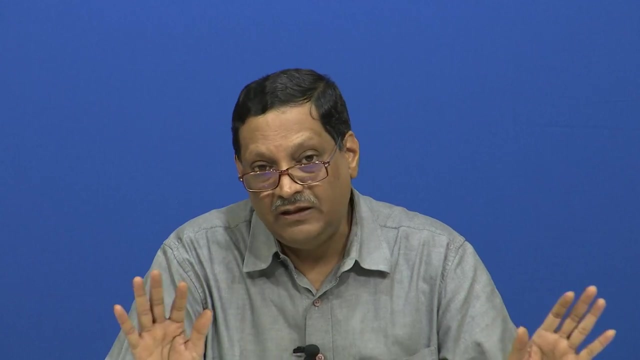 just a lifetime of about a month or two. I will use it, I will ensure it is biodegradable, I will throw it, I will buy a new one and then I will be done. fantastic, right. So you are really revolutionizing the way you are doing air quality measurement every. 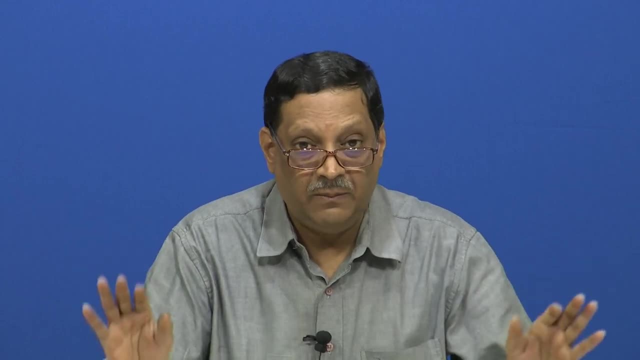 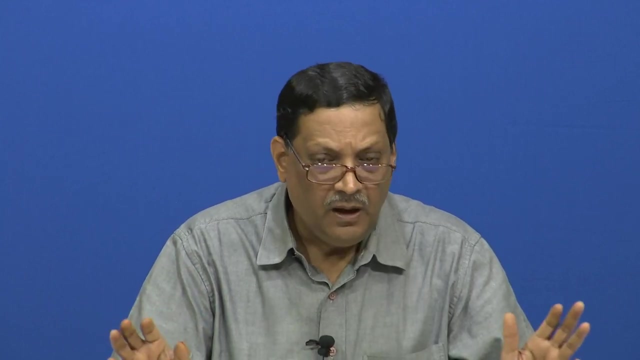 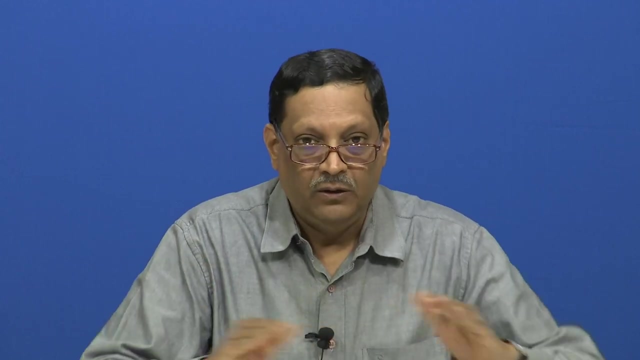 individual around, wherever he or she is making a measurement and sort of, you know, getting some update on what is good, what is bad and so on. but that is a really a dream. it is not going to happen. So, just like that, at least at the household level, if you have a piece of equipment which 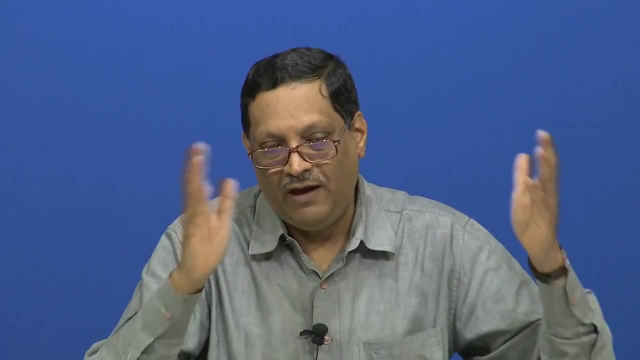 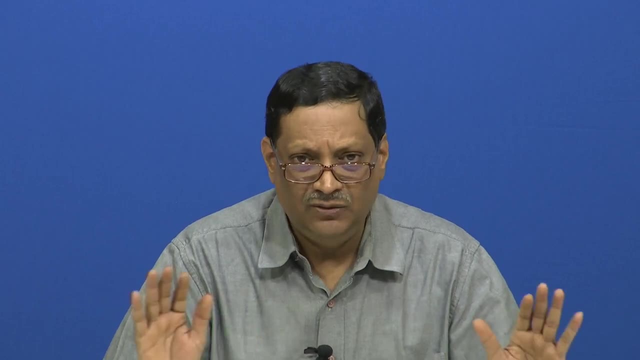 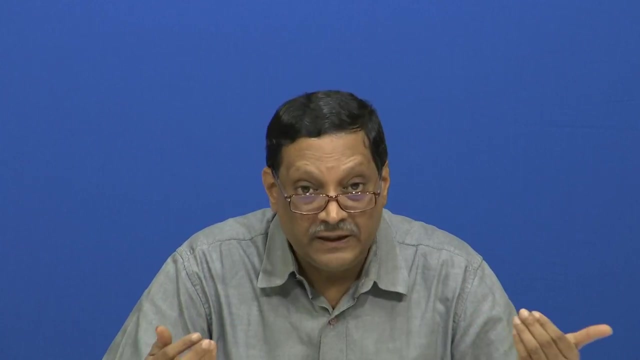 sort of monitors, everything. it is like the wall clock. if you have 1 wall clock equivalent thing for the home and it becomes affordable to buy that device. fantastic, you have done really a wonder. So let us see how to build these systems and what kind of problems technologists have. 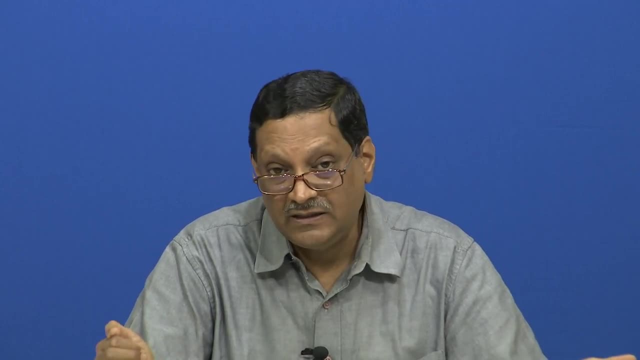 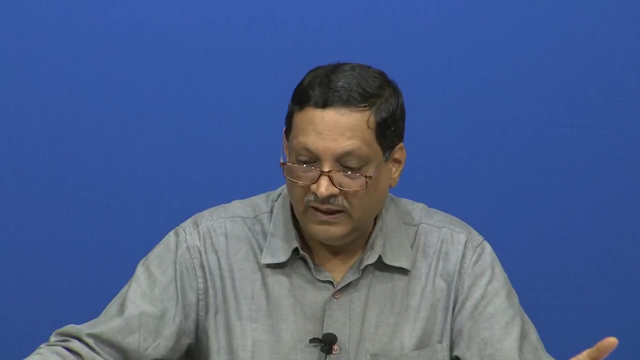 in trying to instrument and they make these systems cheap, affordable. So let us see how to build these systems and what kind of problems technologists have in trying to instrument, and they make these systems cheap, affordable as well, as you know, in simple way, system design such products. so this is one thing. so summary is: you must go back and read. 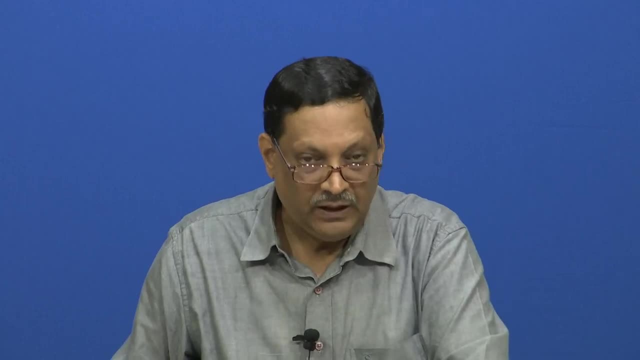 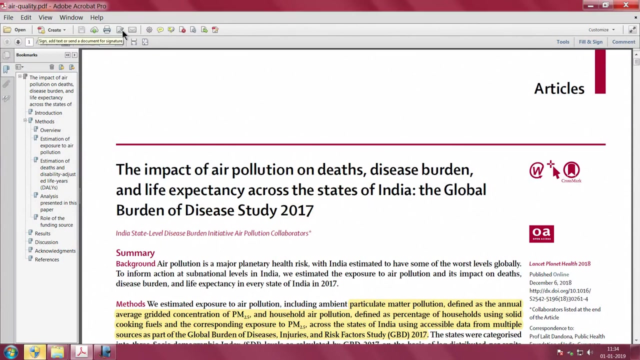 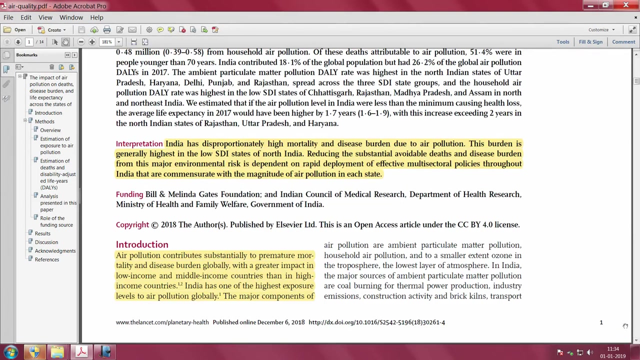 this article. so i will open this article for you and this is the article of interest. reading this article, and let me ensure that we go through this article in a little bit more detail. i have marked some parts of it. i am sure you will be able to. 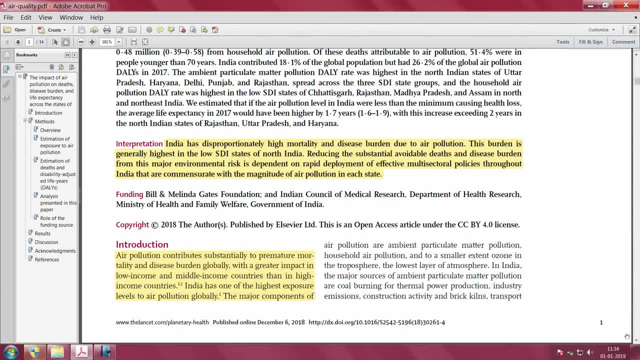 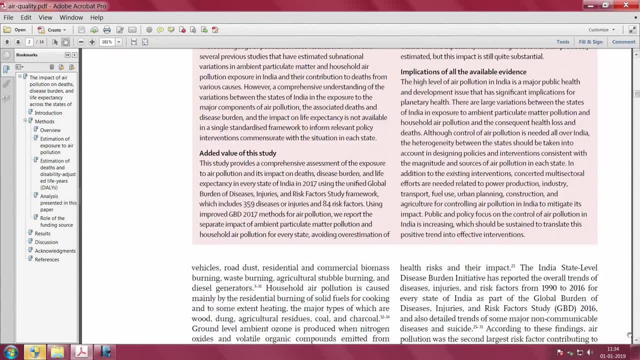 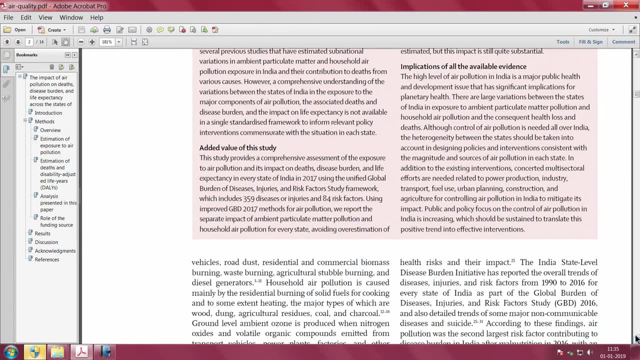 download this article and read it and you know. look at how grim the situation is. so this paper is also talking about how does one arrive at some super conclusions like the ones that we have. this paper is talking about the methodology as well, so it will give you some 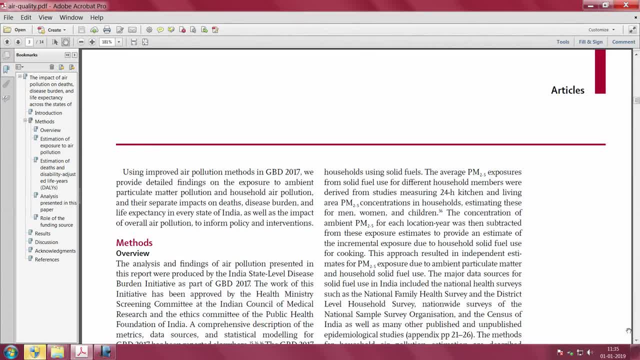 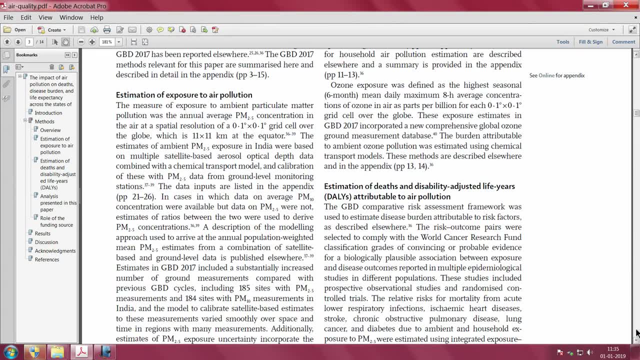 idea on how they went about making that research and how they actually concluded. so the methods in which they have used to estimate. so the methods in which they have used to estimate air exposure, of air pollution: what is the area, what is the grid size and what kind of 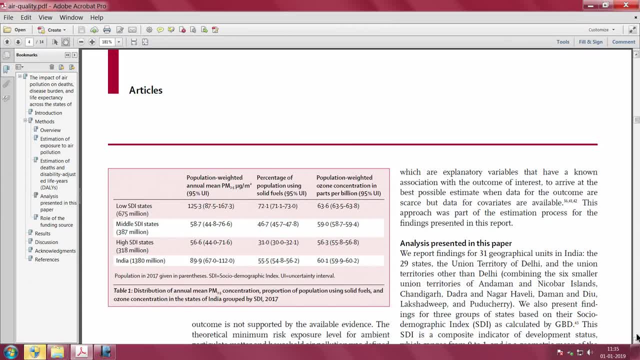 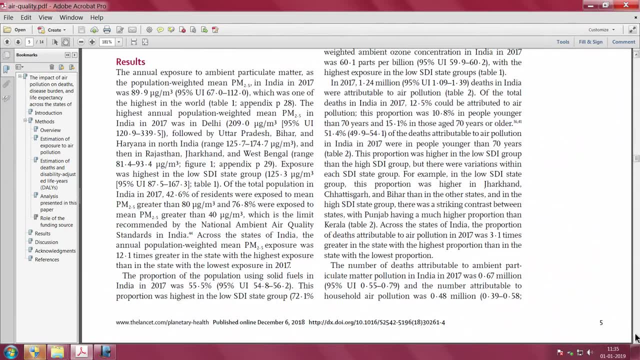 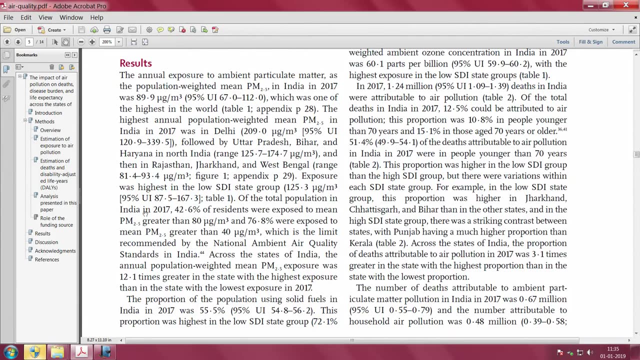 methodology they adapted. all of that is out there in this paper, so we will skip all that, but we will come to the most important part, which is sources. right, you can see here this particular part. it says: of the total population in india in 2017, 42.6 percent of residents were exposed to mean. 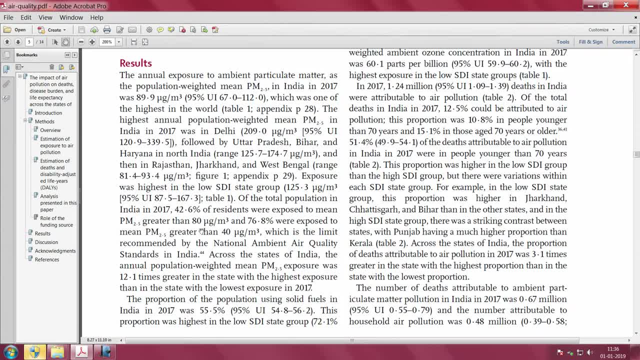 particulate matter 2.5 greater than 80 microgram per meter cube and 76.8 were exposed to mean particulate matter greater than 40 microgram per meter cube, which is the limit recommended by national ambient air quality standards in india. this is indeed the indian standard. then it says: 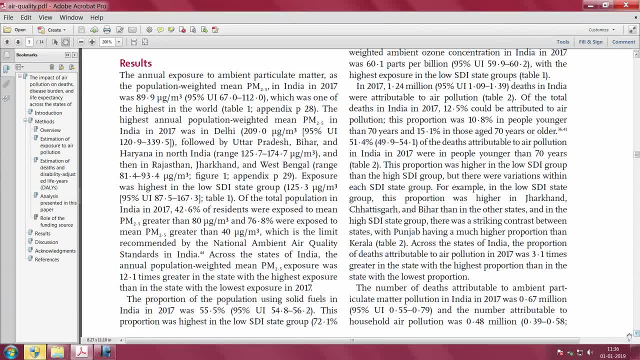 across states. what is the exposure and so on and so forth and the number of deaths that are attributable to ambient pm pollution. are Chip City policies which have broken some of the regulations, at least few countries, and some are established after the Arab articulation: 없는 incenses are inj pas par. 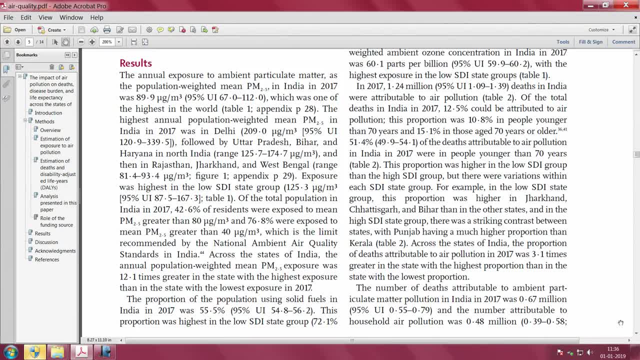 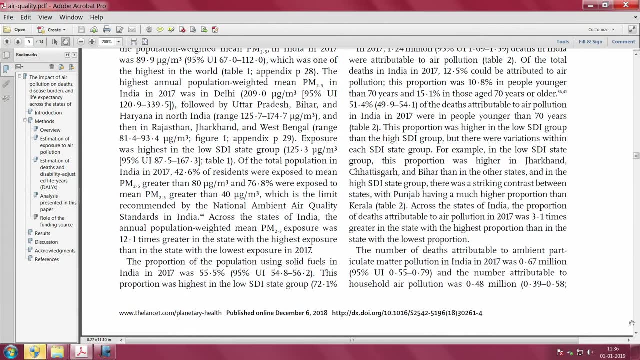 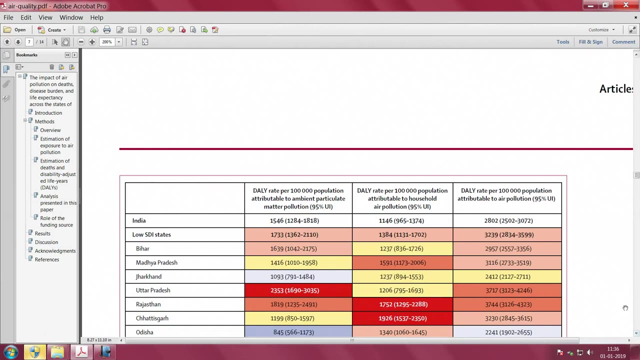 to ambient PM pollution in India is 2017, was some number- 0.67 million- and the number attributable to household air pollution is 0.48 million. So these numbers will keep coming and you have to read it carefully to understand what exactly is the real issue behind this air quality. 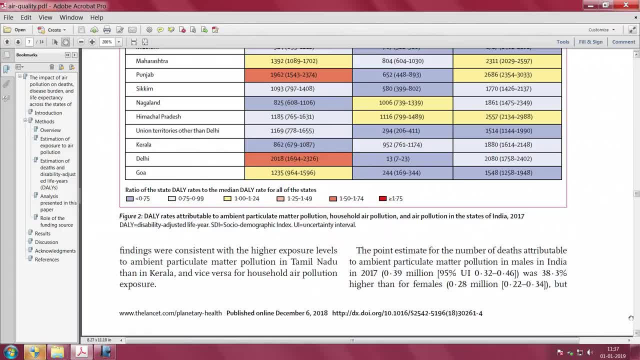 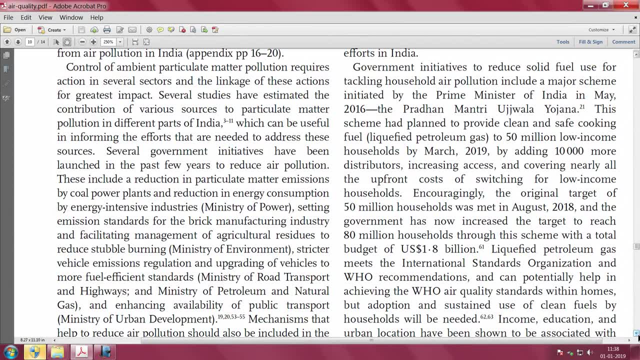 So just to fly through this article. so let us do this reading together and get a grip of the subject. Control of ambient particulate matter. pollution requires several action in several sectors and linkage of these actions for greatest impact- Exactly what we discussed. several studies have estimated the contribution of various 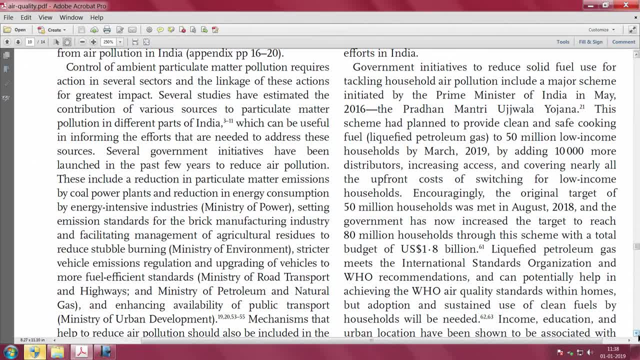 sources of particulate matter pollution in different parts of India, which can be useful in informing efforts That are needed to address these sources. several government initiatives have been launched in the past few years to reduce air pollution. the several efforts have been there and this include reduction. 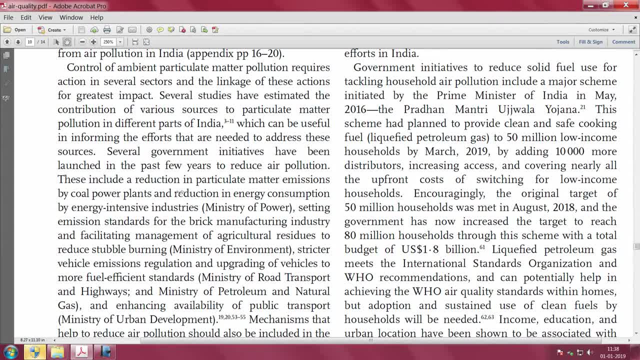 in pm emissions by coal power plants and reduction in energy consumption by energy intensive industries. so first thing, reduction in pm means you should do reduction in particulate matter emissions by coal power plants. our coal power plants, power plants should be much more efficient in its generation and also it should have efficiency in reduction in. 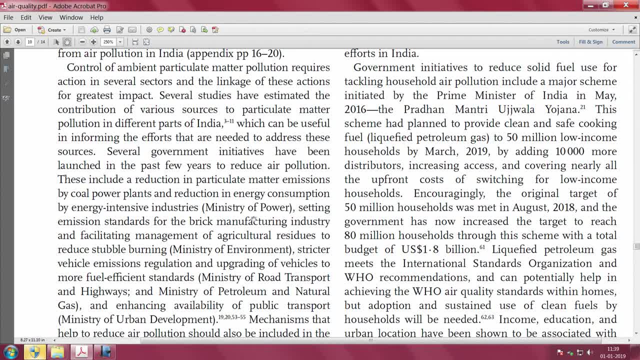 pm emissions. this is what ministry of power is pushing: setting emission standard for the brick manufacturing industry and facilitating management of agricultural residues to reduce stubble burning. this is a become a major issue, 14 In fact. In fact, the problem of Delhi pollution, air quality pollution, indeed is something happening. 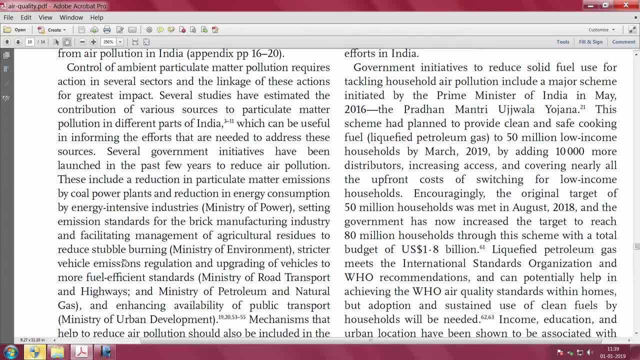 from neighboring states. at least this is what the claim of the Delhi government. So this is the second thing: facilitating management of agricultural residues to reduce stubble burning. So one is coal power plants, second is stubble burning, ministry of environment, stricter vehicle emissions regulation and upgrading of vehicles to more fuel efficient standards. third is 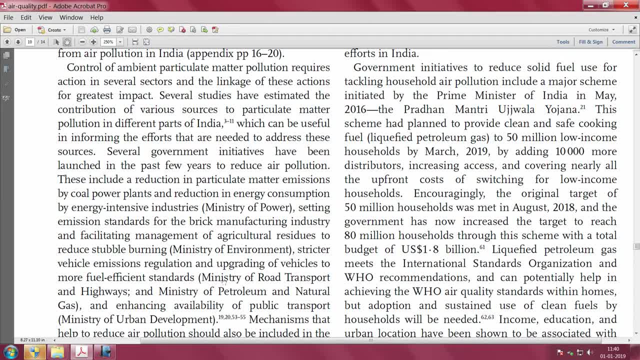 vehicular pollution right, and that is from ministry of road transport and highways and ministry of petroleum and natural gas, and the other one is an enhancing availability of public transport. when you do mass transport of people, you are bound to reduce the number of fossil fuel driven vehicles and therefore public transport. ministry of urban development. 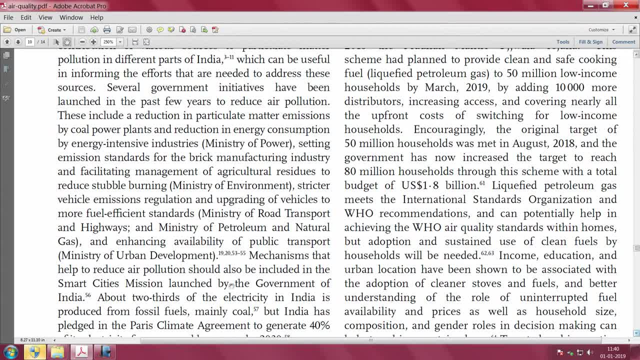 right So on. mechanisms that help reduce air pollution should be included in the smart cities mission launched by government of India. about two-thirds of electricity in India is produced from fossil fuels, mainly coal. see, it is again back to coal, but India has pledged in the Paris climate. 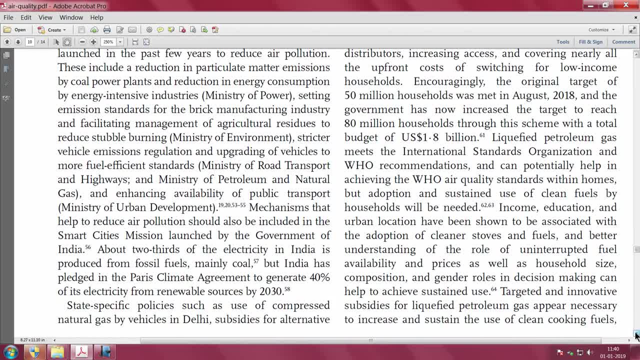 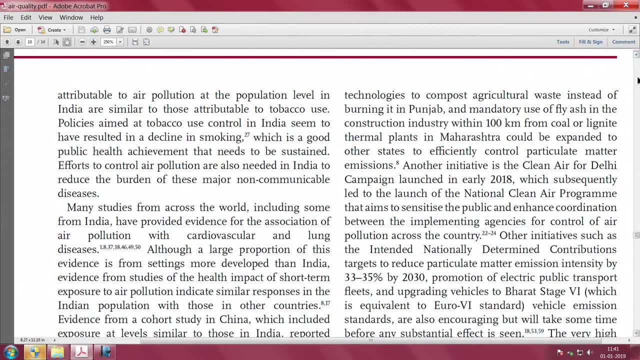 agreement to generate 40 percent of its electricity from renewable sources by some year 2030. state specific policies, such as compressed natural gas. So these are some of the mechanisms that can be used to reduce the number of fossil fuels that are produced by vehicles in Delhi. subsidies for alternative technologies to 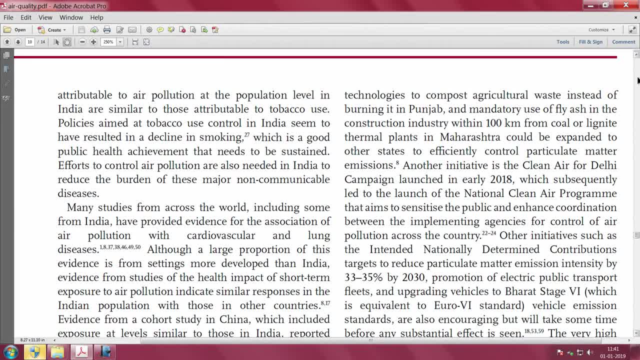 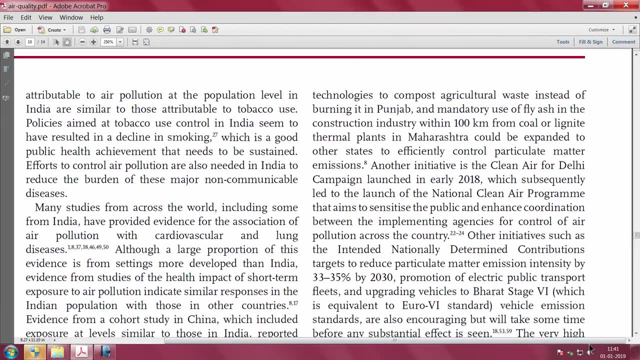 compost agricultural waste instead of burning it in Punjab and mandatory use of fly ash in the construction industry within 100 kilometer from coal or lignite thermal plants in Maharashtra could be expanded to other states to efficiently control particulate matter emissions. So there are mitigation mechanisms which are looking at how to manage particulate matter. 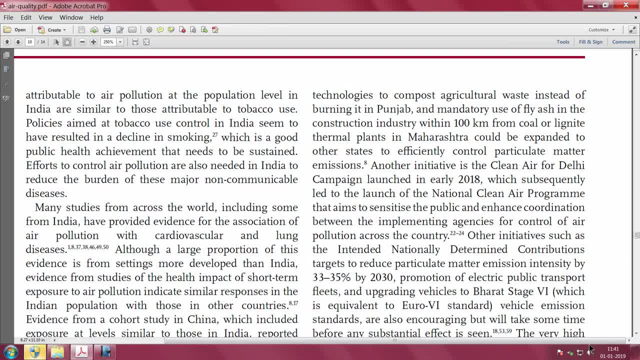 itself So that you have clean air. another initiative is the clean air for Delhi campaign, launched in early 2018, which subsequently to launch national clean air program that aims to sensitize public and enhance coordination between implementing agencies for control of air pollution, and so on. 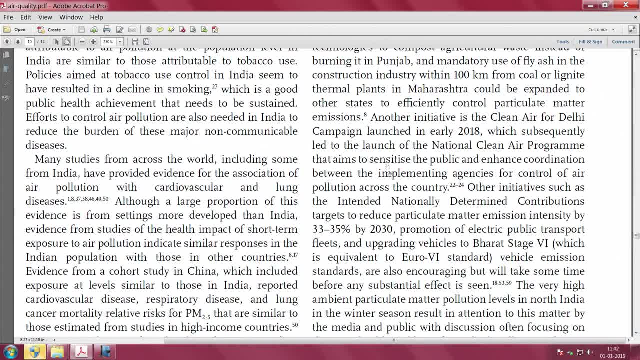 So then there is other initiatives, such as intended nationally determined contributions. targets to reduce PM emissions by 33 to 35 percent By 2030, promotion of electric public transport fleets, upgrading vehicles to barrage stage 6, which is equivalent to Euro 6 standard vehicle emission standards are also encouraging. 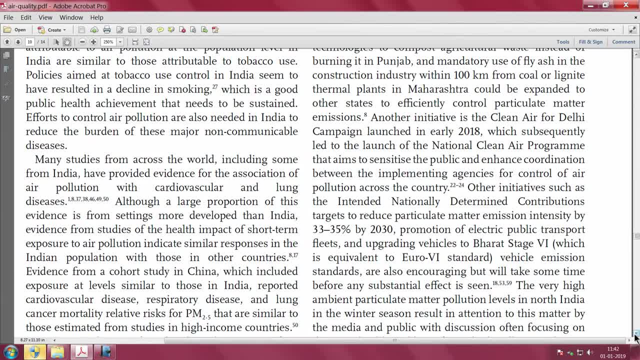 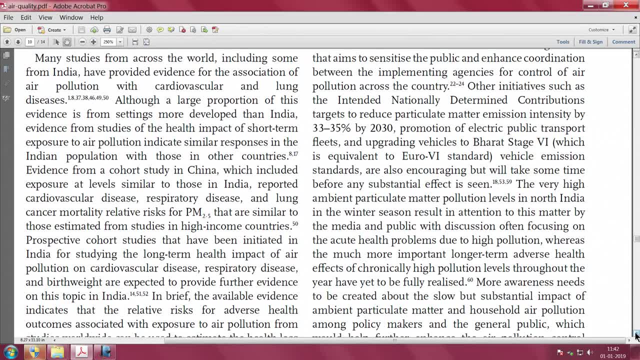 but will take some time before any substantial effect is seen. So you can see so many reasons why particulate matter is an issue. coal fired right coal is an issue, Then stubble burning is another issue, then vehicular emissions is an issue per generation. 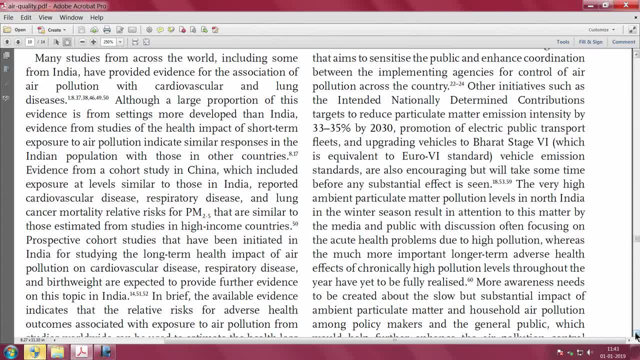 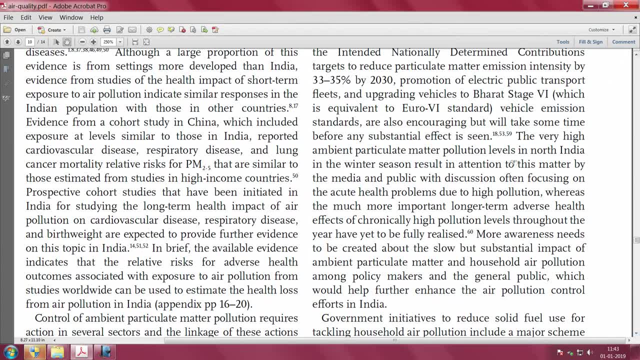 of particulate matter and all that. So the fourth one indeed also we will come to. so we have already identified three in the very high ambient particulate matter pollution levels in North India in the winter season result in attention to this matter by the media and public, with discussion on focusing 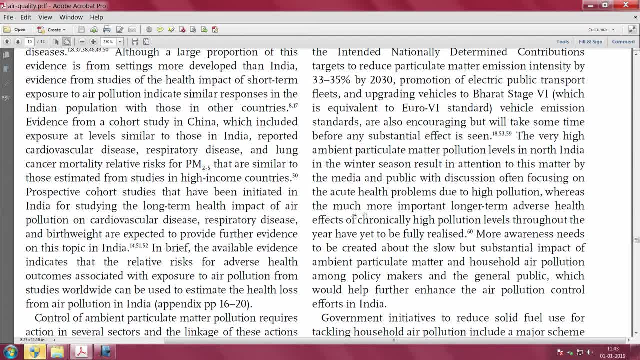 on the acute health problems due to high pollution, As the much more important longer term adverse health effects of chronically high pollution levels throughout the year have yet to be fully realized. more awareness needs to be created about this low but substantial impact of ambient particulate matter and household. 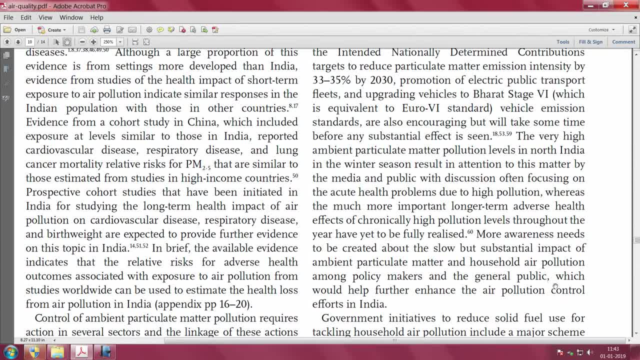 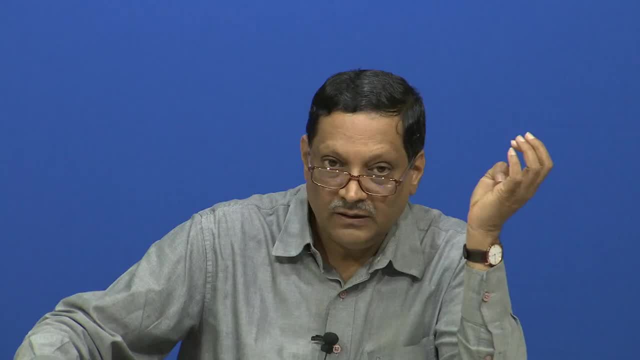 air pollution among policy makers and the general public, which would help further enhance the air pollution control efforts in India. So you can see, household air pollution is another major. So how many we have identified already? coal fired power plants, stubble burning. third, 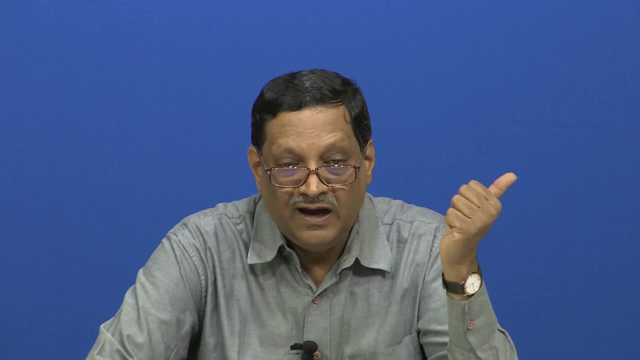 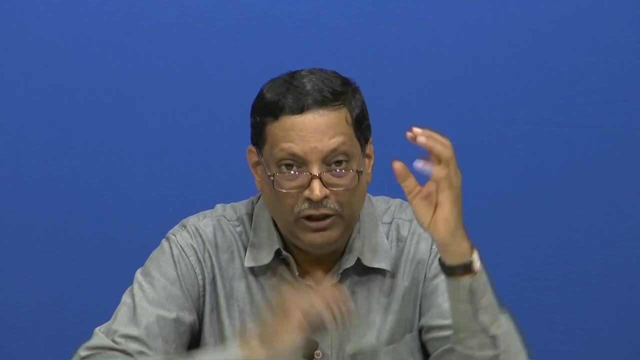 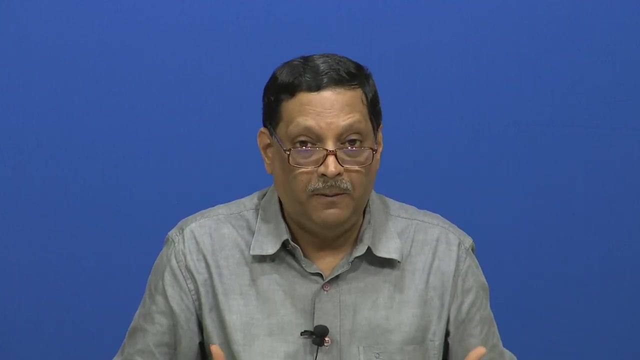 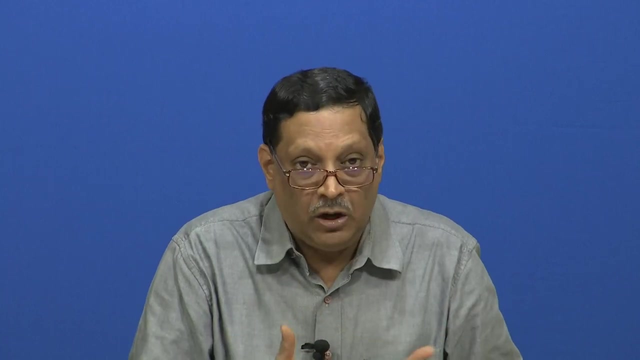 one is vehicular emissions. fourth one is household air pollution. four major, four major bullets. if you have to say who generates what generates particulate matter, you can think of these four as a major problem and you have to control each one of them As much as possible and you have to monitor first. if you have to control, you have to monitor. 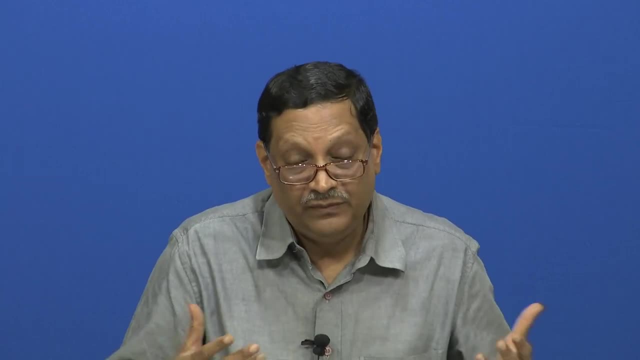 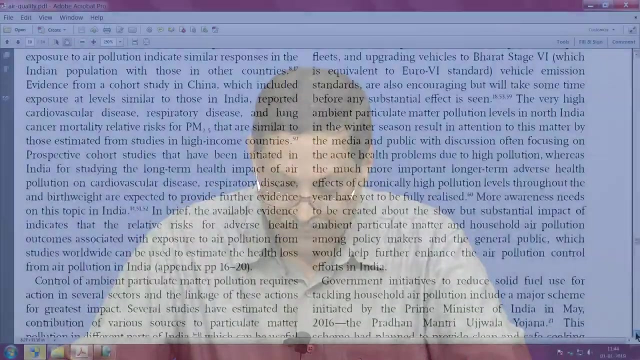 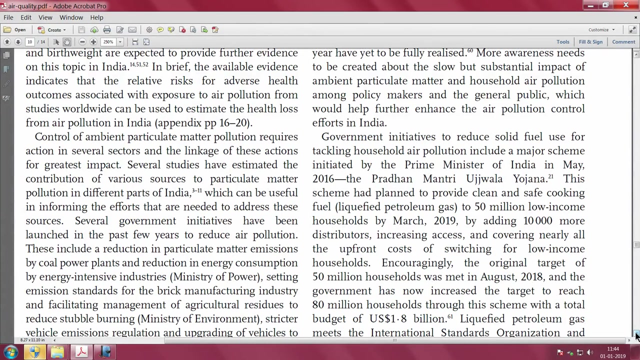 right. So you have to do sensing. So the large scale sensing, then followed by some actuation, some control, Come to household air pollution. government initiatives to reduce solid fuel use, tackling household air pollution, include a major scheme. You know about the Pradhan Mantri Ujjwala Yojana, which was started in 2016,. it is trying 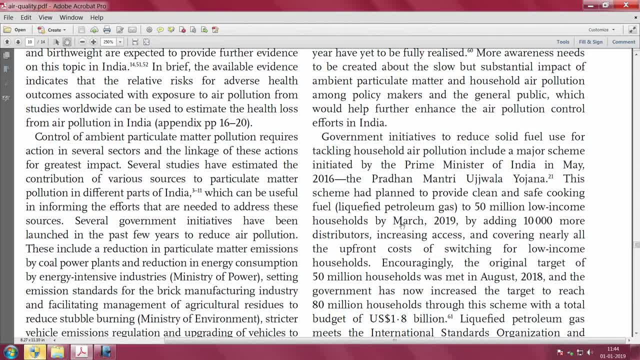 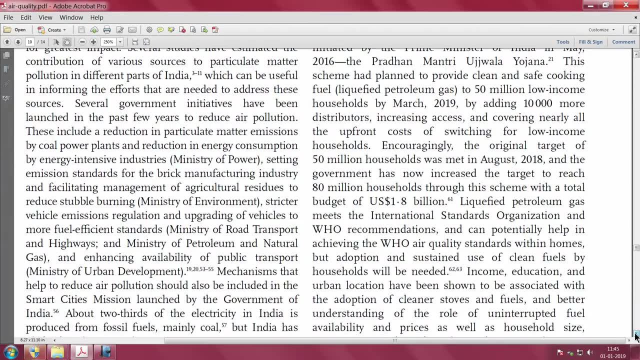 to provide clean and safe Cooking fuel, liquefied petroleum gas, to 50 million low income households by some year, by adding 10,000 more distributors and trying to giving access clean fuel and also, essentially, all of this means that you know you have to move in the direction of sense and mitigate. 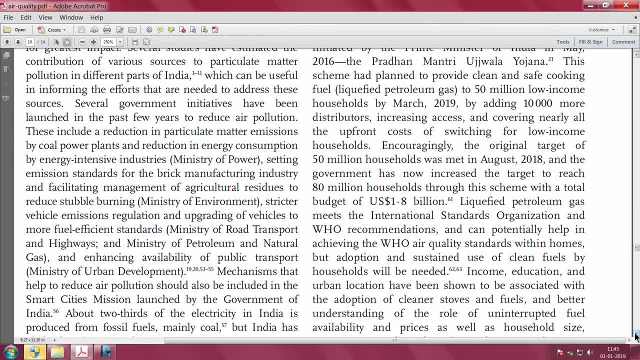 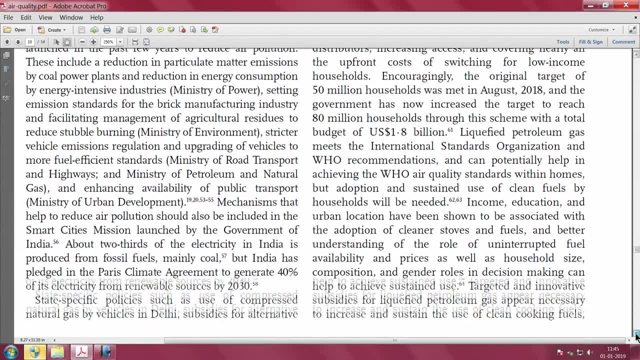 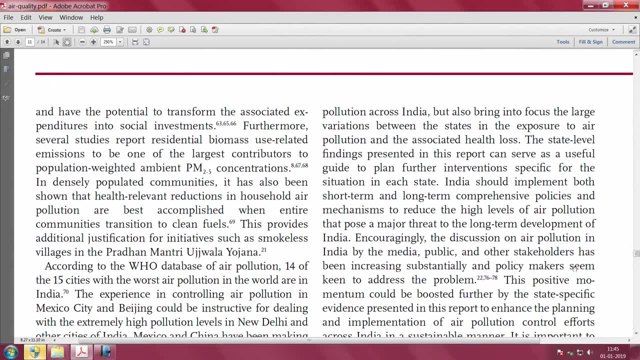 reduce particulate matter. The WHO air quality standard within homes Is there and you have to adhere to those WHO recommendation so that you essentially keep the pollution levels at the manageable levels. There are several studies that reports as residential biomass use related emissions to be one of the largest contributors of population weighted ambient PM 2.5 concentrations. 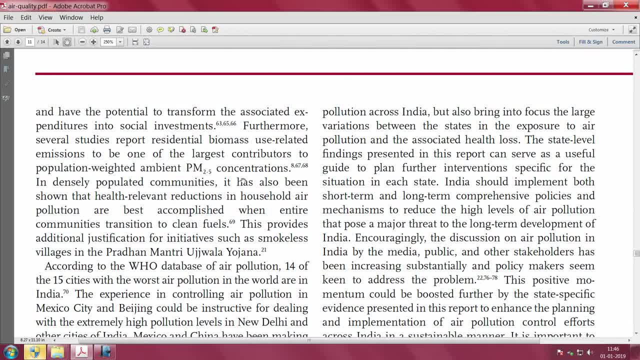 So in densely populated communities. it has also been shown that health relevant reductions in household air pollution Are best accomplished when entire communities transition to clean fuel. it is not enough if you do in one, So you have to do it in a major way. smoke less villages. in all that you have to worry. 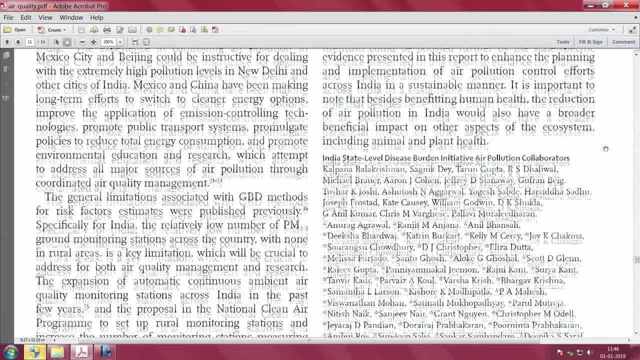 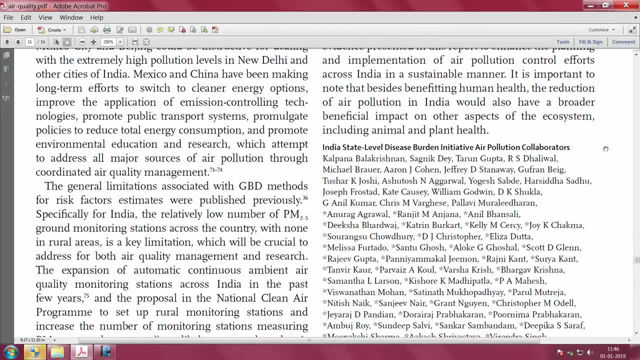 about. So, essentially, I want you to read this paper in a great detail and arrive at you know your own conclusion on why this is a huge problem And what we can do to reduce, to monitor using IOT. So, essentially, I want you to read this paper in great detail and arrive at you know your 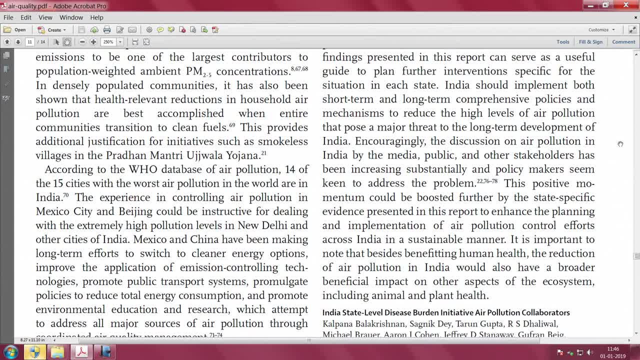 own conclusion on why this is a huge problem And what we can do to reduce, to monitor using IOT. So, essentially, I want you to read this paper in a great detail and arrive at, you know, your own conclusion on why this is a huge problem. 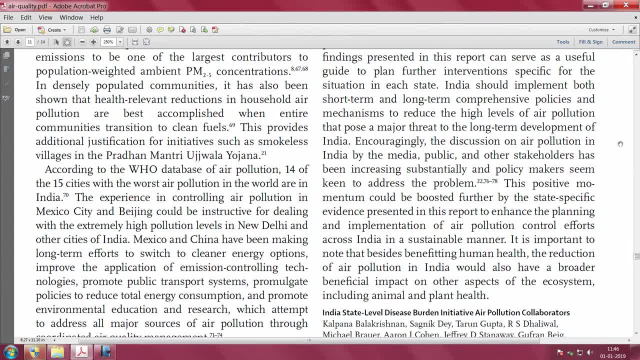 And what we can do to reduce to monitor using IOT. So, essentially, I want you to read this paper in a great detail and arrive at, you know, your own conclusion on why this is a huge problem And what we can do to reduce to monitor using IOT. 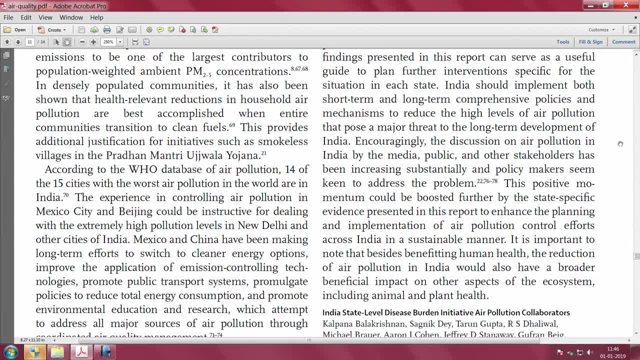 So, essentially, I want you to read this paper in a great detail and arrive at you know your own conclusion on why this is a huge problem And what we can do to reduce, to monitor using IOT. So, essentially, I want you to read this paper in a great detail and arrive at you know your. 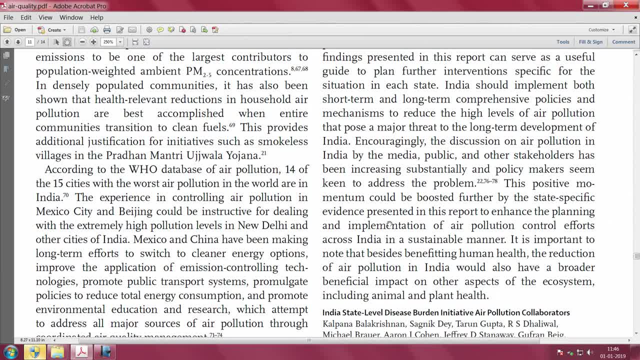 own conclusion on why this is a huge problem And what we can do to reduce, to monitor using IOT. So, essentially, I want you to read this paper in a great detail and arrive at, you know, your own conclusion on why this is a huge problem. 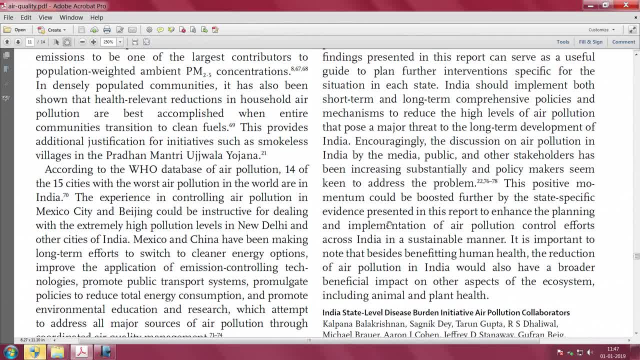 And what we can do to reduce to monitor using IOT. So, essentially, I want you to read this paper in a great detail and arrive at, you know, your own conclusion on why this is a huge problem And what we can do to reduce to monitor using IOT. 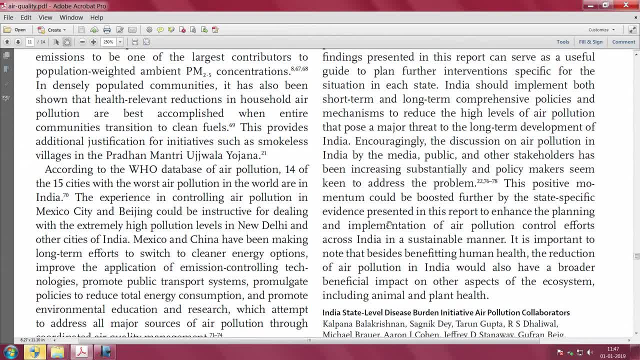 So, essentially, I want you to read this paper in a great detail and arrive at you know your own conclusion on why this is a huge problem And what we can do to reduce, to monitor using IOT. So, essentially, I want you to read this paper in a great detail and arrive at you know your. 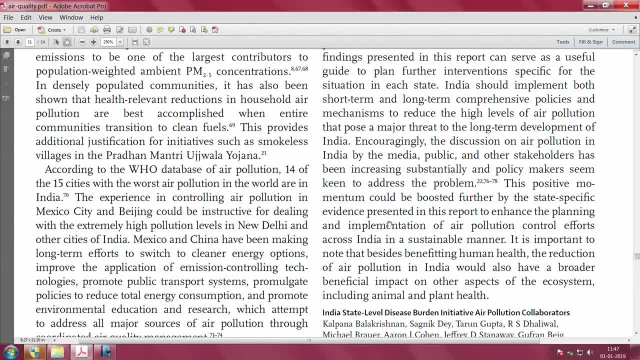 own conclusion on why this is a huge problem And what we can do to reduce, to monitor using IOT. So, essentially, I want you to read this paper in a great detail and arrive at, you know, your own conclusion on why this is a huge problem. 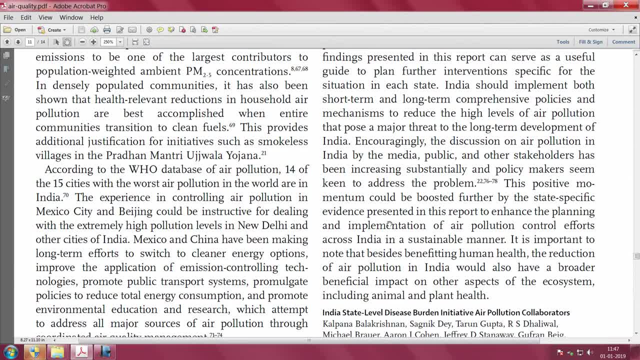 And what we can do to reduce to monitor using IOT. So, essentially, I want you to read this paper in a great detail and arrive at, you know, your own conclusion on why this is a huge problem And what we can do to reduce to monitor using IOT. 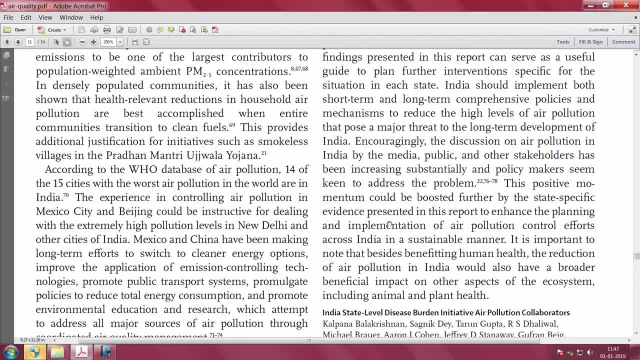 So, essentially, I want you to read this paper in a great detail and arrive at you know your own conclusion on why this is a huge problem And what we can do to reduce, to monitor using IOT. So, essentially, I want you to read this paper in a great detail and arrive at you know your. 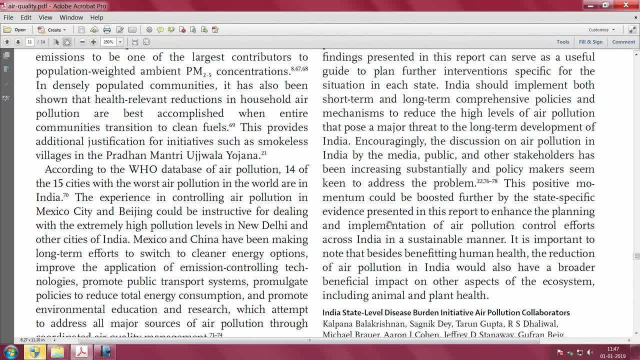 own conclusion on why this is a huge problem And what we can do to reduce, to monitor using IOT. So, essentially, I want you to read this paper in a great detail and arrive at, you know, your own conclusion on why this is a huge problem. 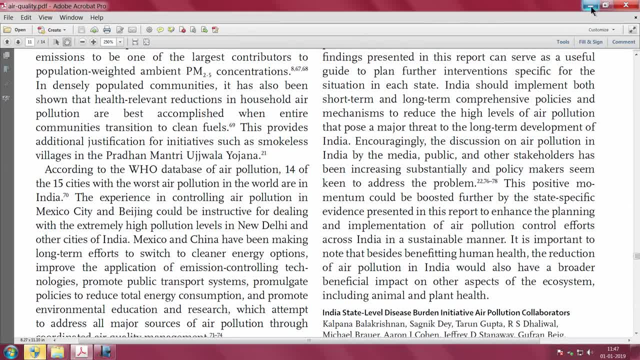 And what we can do to reduce to monitor using IOT. So, essentially, I want you to read this paper in a great detail and arrive at, you know, your own conclusion on why this is a huge problem And what we can do to reduce to monitor using IOT. 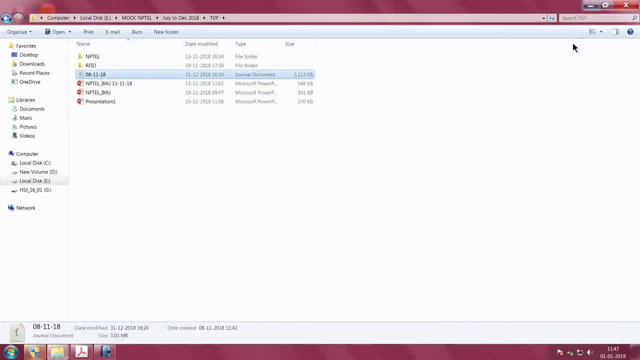 So, essentially, I want you to read this paper in a great detail and arrive at you know your own conclusion on why this is a huge problem And what we can do to reduce, to monitor using IOT. So, essentially, I want you to read this paper in a great detail and arrive at you know your. 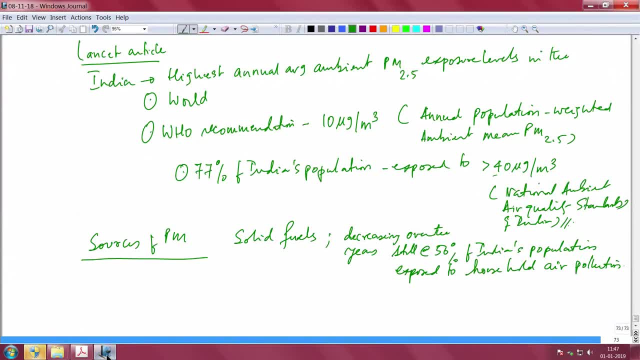 own conclusion on why this is a huge problem And what we can do to reduce, to monitor using IOT. So, essentially, I want you to read this paper in a great detail and arrive at, you know, your own conclusion on why this is a huge problem. 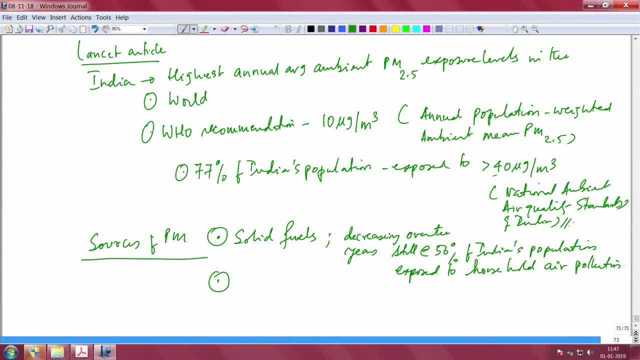 And what we can do to reduce to monitor using IOT. So, essentially, I want you to read this paper in a great detail and arrive at, you know, your own conclusion on why this is a huge problem And what we can do to reduce to monitor using IOT. 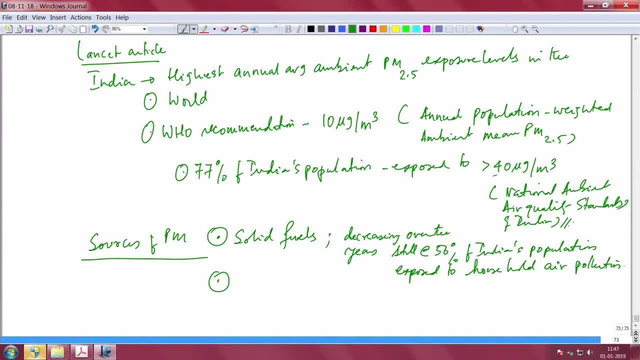 So, essentially, I want you to read this paper in a great detail and arrive at you know your own conclusion on why this is a huge problem And what we can do to reduce, to monitor using IOT. So, essentially, I want you to read this paper in a great detail and arrive at you know your. 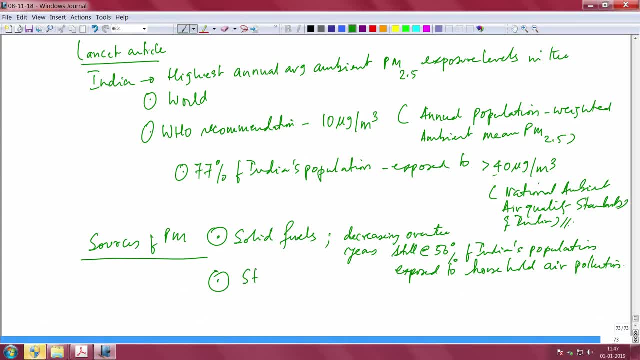 own conclusion on why this is a huge problem And what we can do to reduce, to monitor using IOT. So, essentially, I want you to read this paper in a great detail and arrive at, you know, your own conclusion on why this is a huge problem. 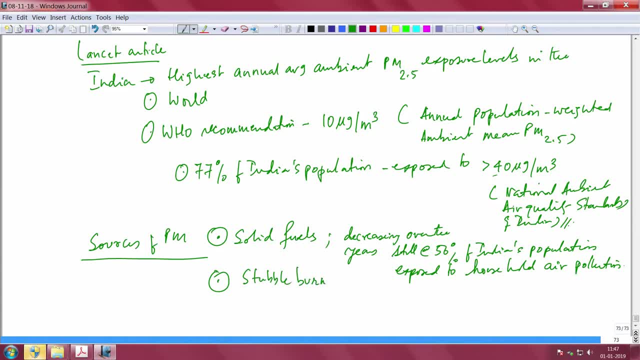 And what we can do to reduce, to monitor using IOT. So, essentially, I want you to read this paper in a great detail and arrive at, you know, your own conclusion on why this is a huge problem. right, This is agricultural residue. Third, transportation: right, This is all about vehicle. 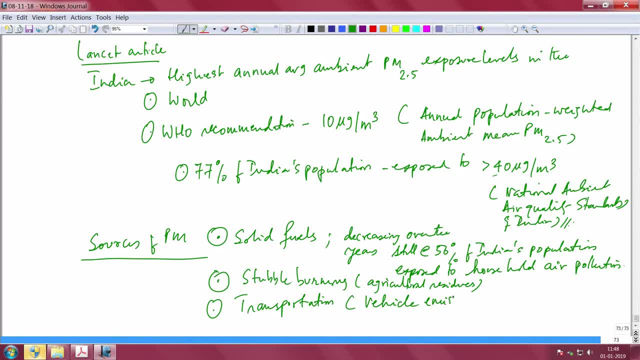 emissions. So solid fuels, stable burning, transportation and energy sector. energy generation sector, generation coal fired plants For the purpose of energy. I would say that you should replace, and then you say solid fuels. How can IOT solve this problem? This is the issue. What I suggest for the remaining? 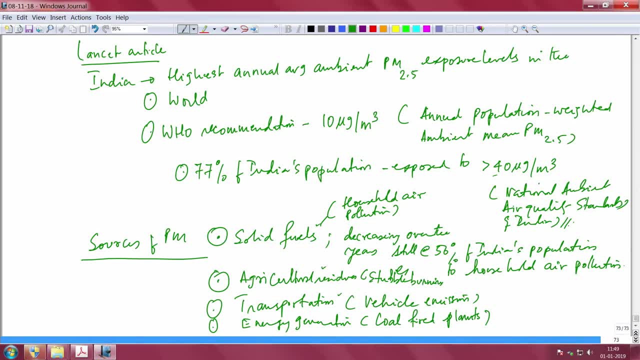 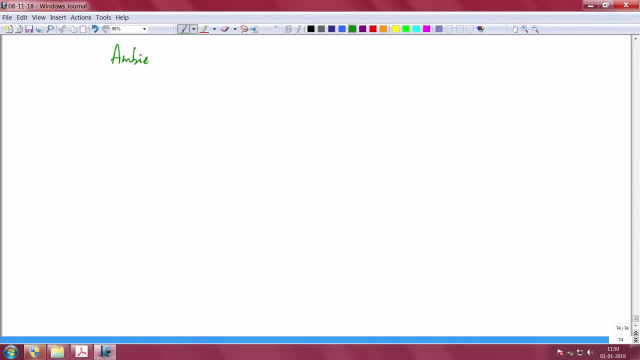 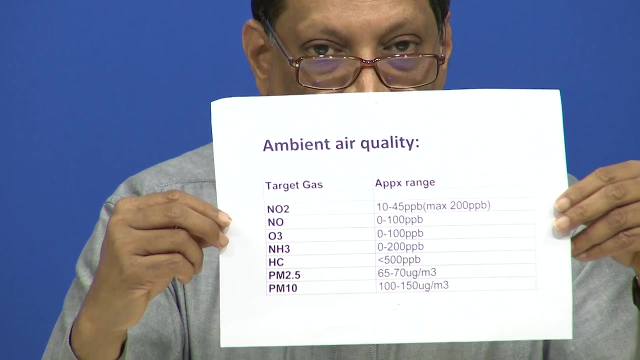 part in this course, rather in this module. ultimately, we have to build systems right. Let us look at ambient air quality and also let us look at vehicle emissions. So I mentioned to you about ambient air quality. I will put back this chart for you. You can read some numbers. 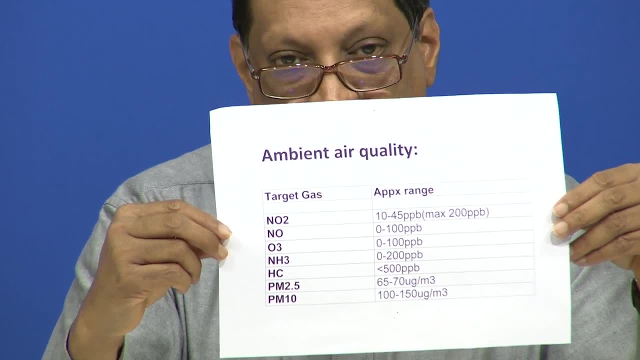 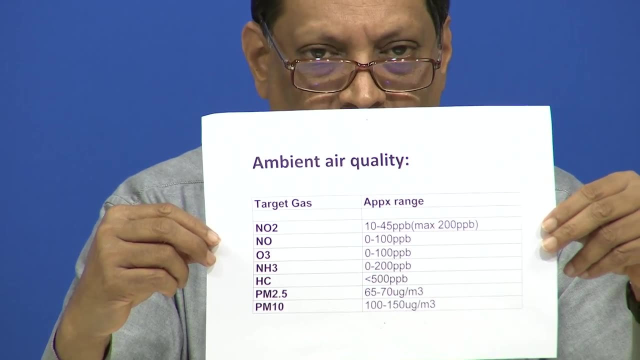 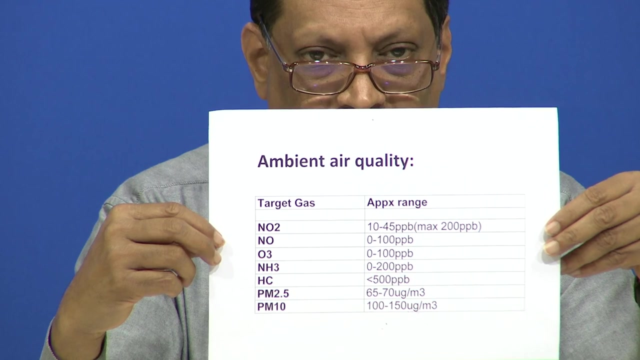 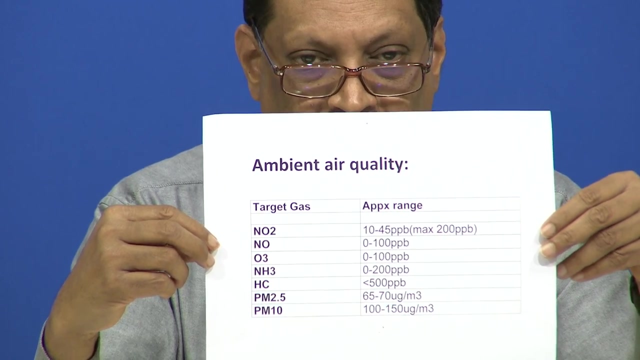 You can see ambient air quality. these are important. There are others. This is adjusted. surrounding air quality and quality. There is sulfur dioxide, for instance. who is missing in this? But nevertheless, nitrogen dioxide is the range. here is the number. here We can see: nitric oxide is mentioned. overstome is mentioned, NH3, ammonia is mentioned. then 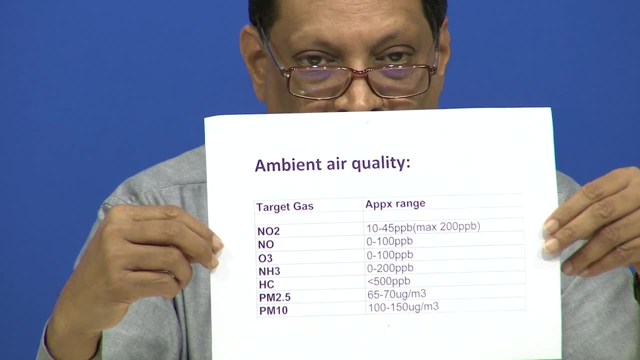 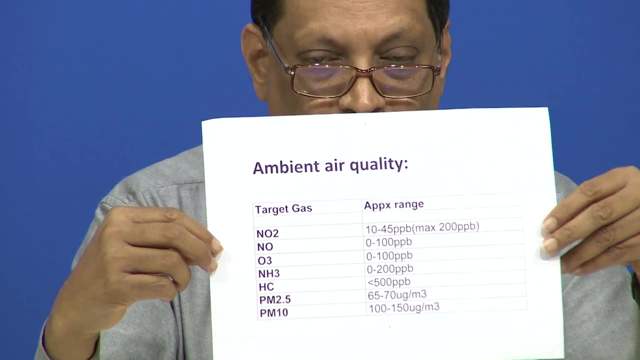 hydrocarbon is mentioned, Particulate matter 2.5 is concerned and particulate matter 10 is mentioned. So for thumbs, coloured paradise or wiring clean-up environment if you wanted to be safe. So you do need to carry a colleague and if you need anything else you do need to. 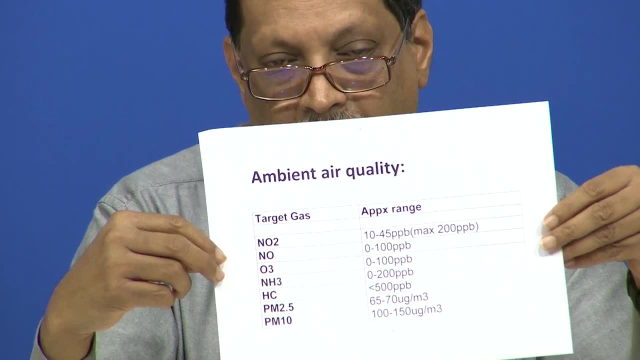 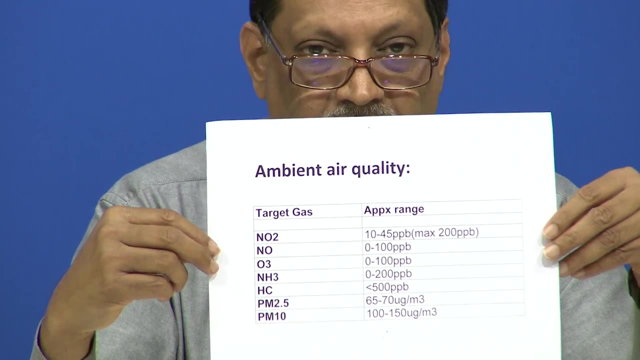 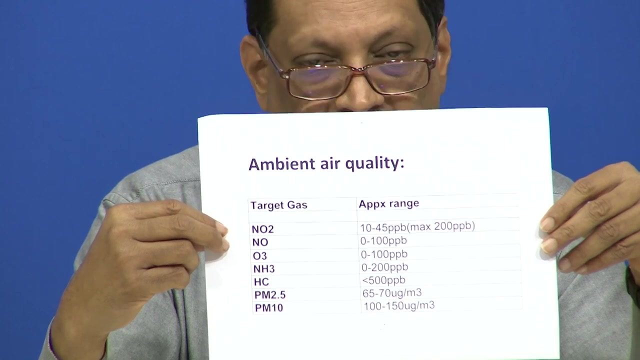 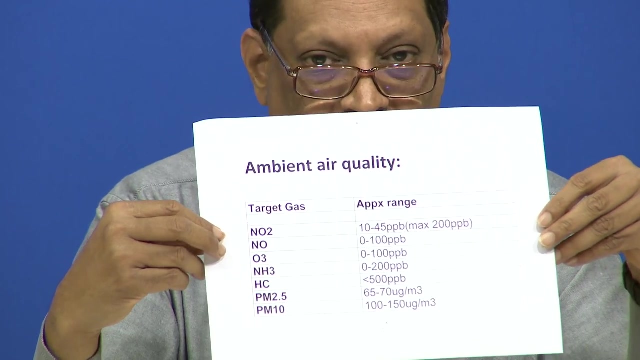 see that 40 microgram per meter cube is what the you know, the safe value which is proposed by Indian standard. but I have put here 65 to 70, which is already extremely bad. no choice at the moment. if you are able to measure 65- 70 microgram per meter cube, you are already. 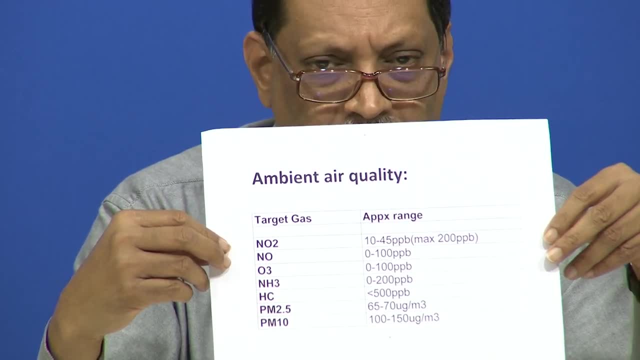 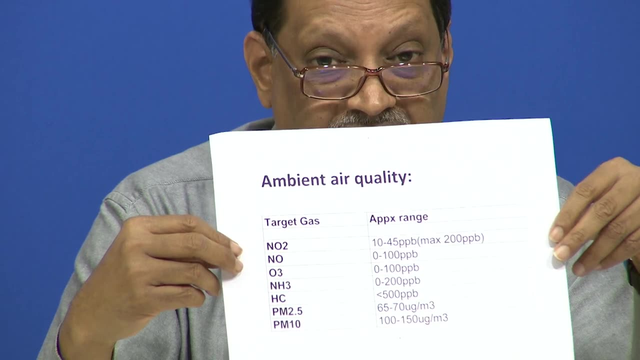 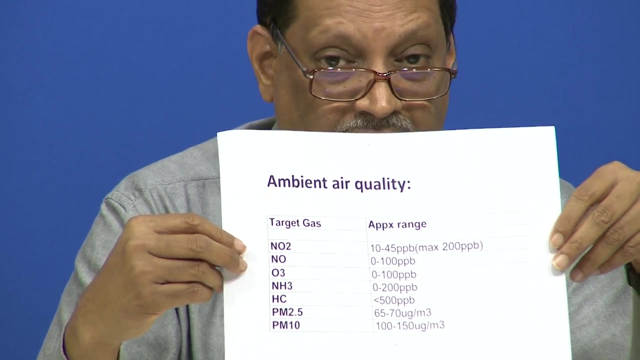 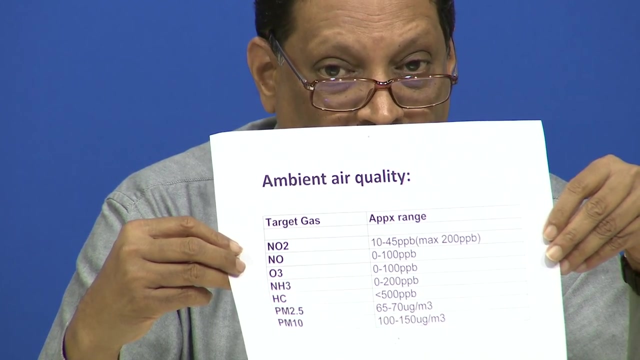 ok, but if this number goes some 4 times higher, you can think that most dangerous pollution level. So where is 10, where is 40 and what is the number I have put here? it sounds pretty ridiculous, but I would say that if you are able to at least monitor this value, 65, 70 microgram per. 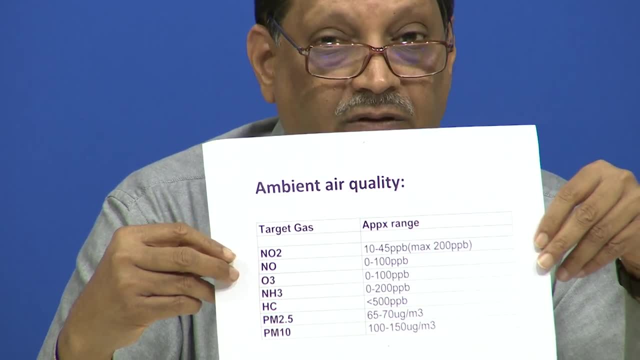 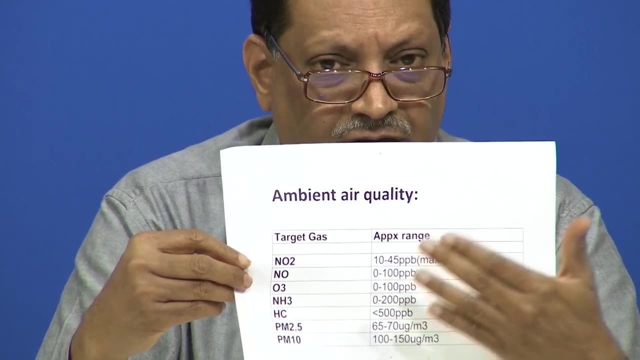 meter cube up to this value accurately, then you are very good. So this is not really. you do not. you do not have to regard this as the number that is very good for humans. it is not a good number for humans. what we are saying is: this is the. 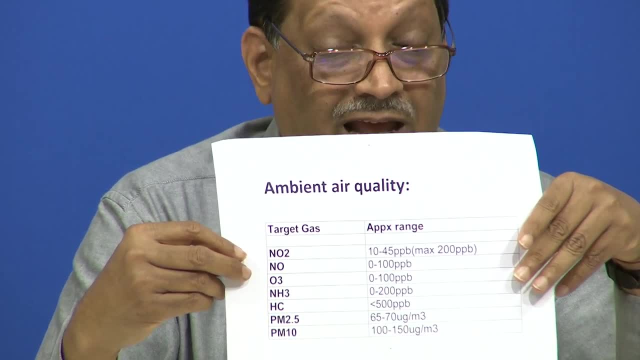 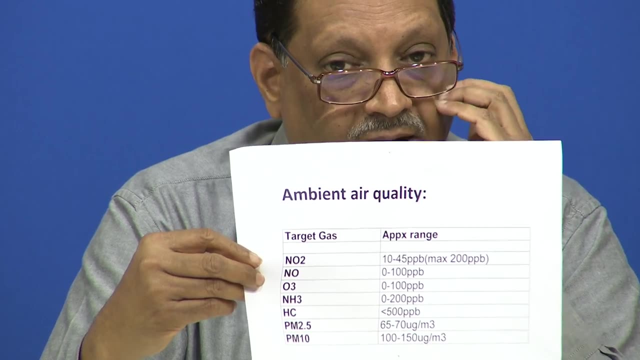 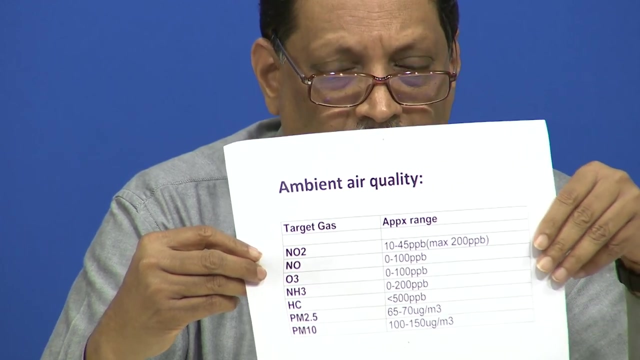 approximate range. you want to measure very accurately. up to this value. you want to measure very accurately, For instance, NO2: 10 to 45 p pb is what it should be even less than that. ok, it should be around 10, 20 p p b or so. 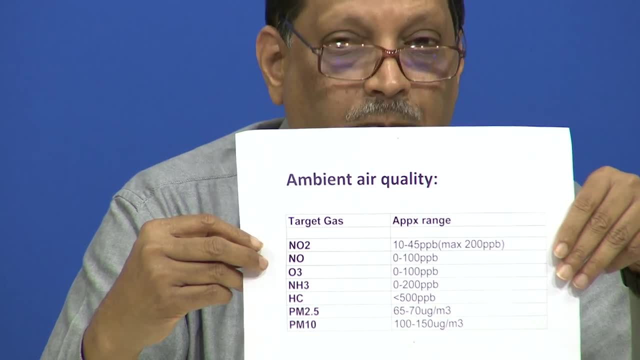 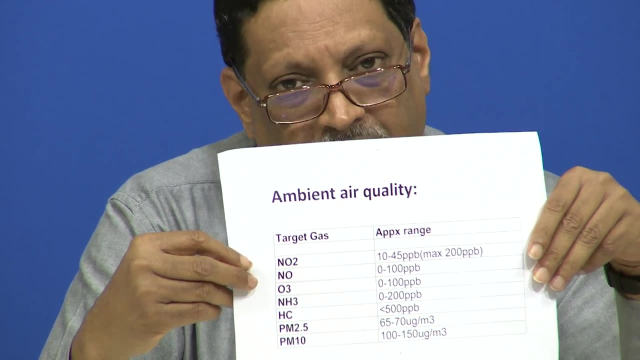 But if you are able to maximum, able to measure up to 200 ppb accurately, whichever sensor you choose, if it is doing that, it is a good job. So kindly interpret this chart more: from the sensor, the sensitivity, the range over. 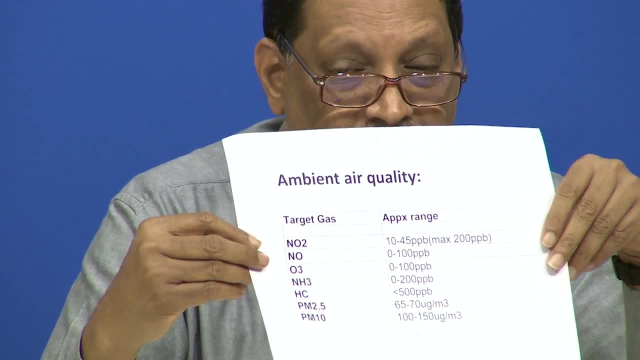 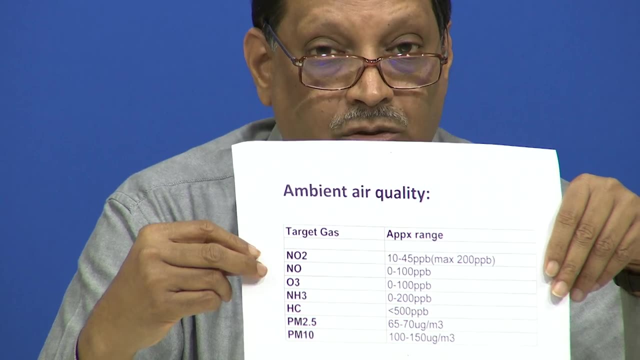 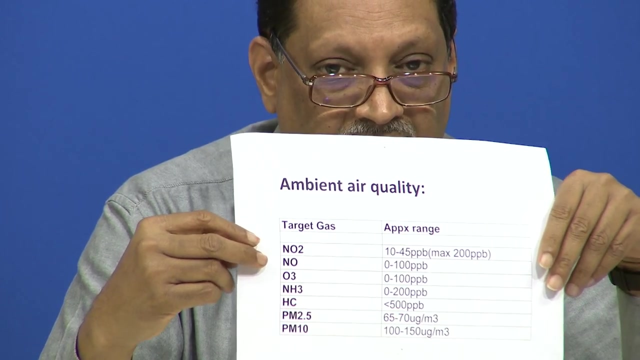 which a sensor should be able to measure these values accurately, not so much from the fact that these are safe values for humans to live in. These are not really safe values for humans to live in And, as you can see, it is a clear indicator- is particulate matter. 2.5, Indian standard. 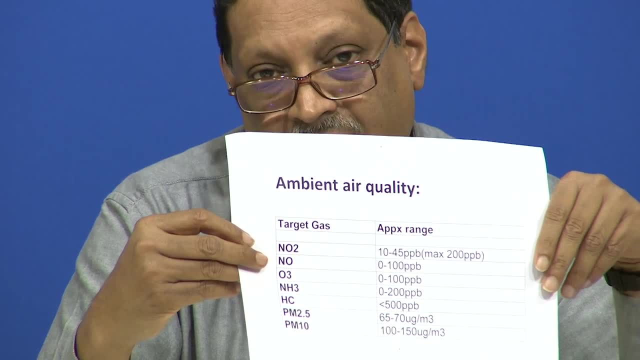 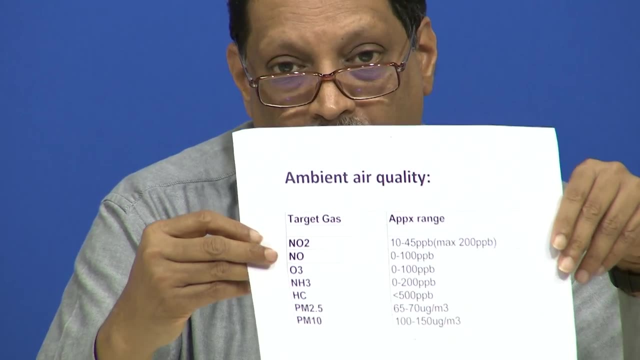 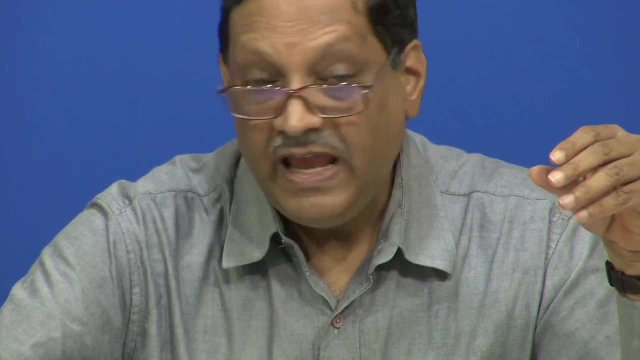 says 40 microgram per meter cube. WHO standard says 10 microgram per meter cube. This is already the difference. So I hope you are clear with the interpretation of this, For a similar chart can also be done for exhaust air quality. 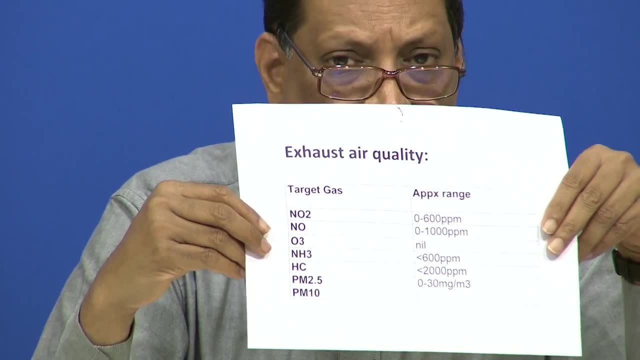 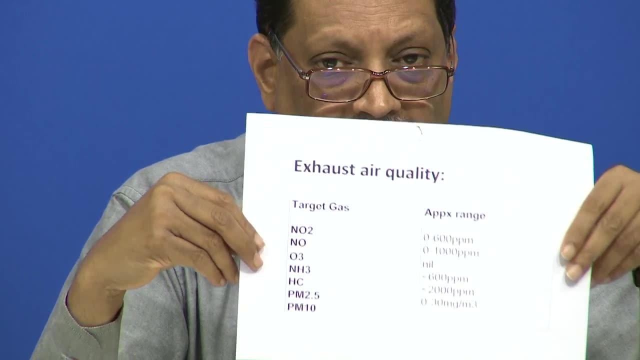 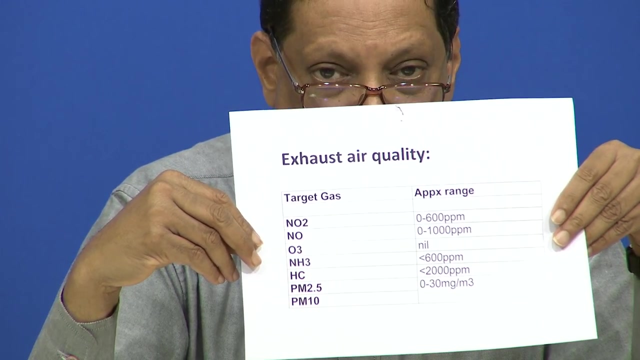 So this is. So this is another problem that we have, And you are looking at sensors which can measure accurately NO2, nitric nitrogen dioxide up to 600 ppm. nitric oxide- up to about 1000 ppm ozone should not be there at all ammonia. 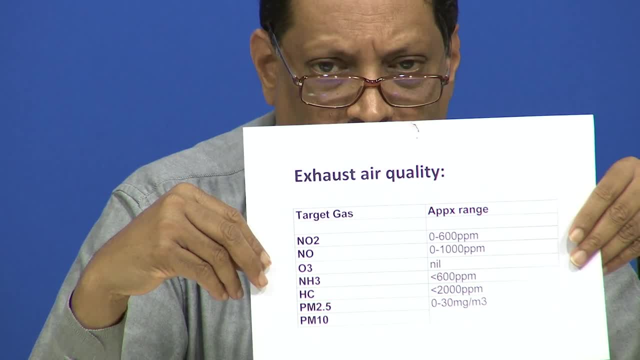 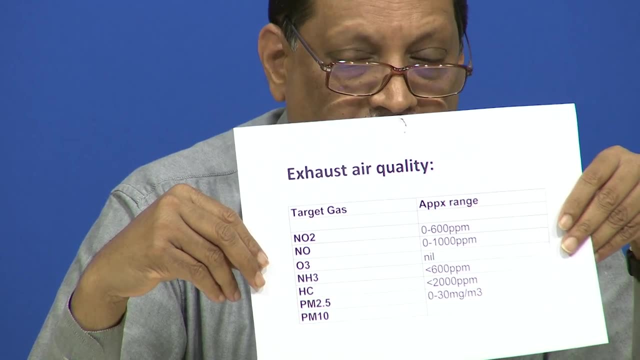 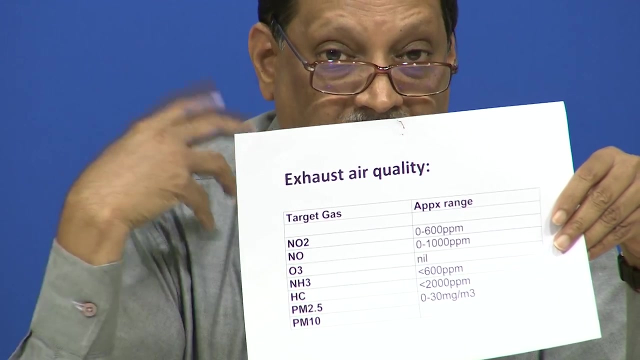 should be less than 600 parts per million and you can see that particulate matter 2.5,. you should be able to measure accurately up to about 30 milligram per meter cube. All this happening because of fuel burning inside the vehicle. 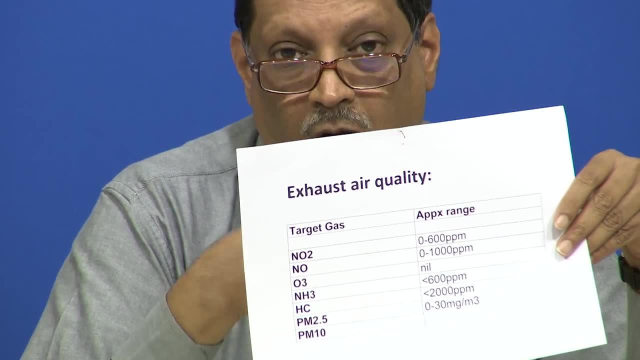 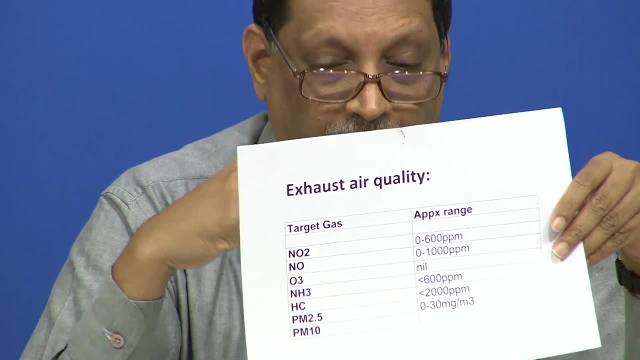 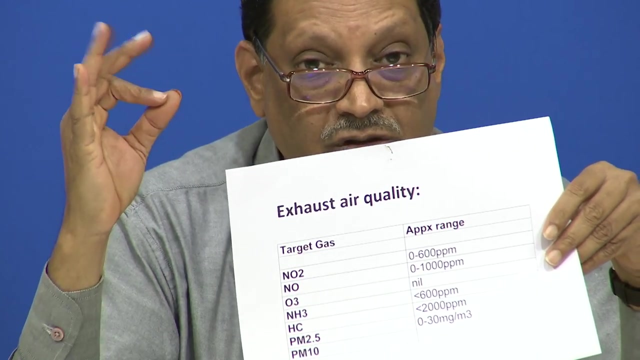 It is all about fossil fuels. it is about petrol, petroleum products like petrol, diesel and so on, which essentially are contributing to these gases which are coming from the tail pipe, Again absolutely unsafe for human breathing. but sensors you choose should essentially